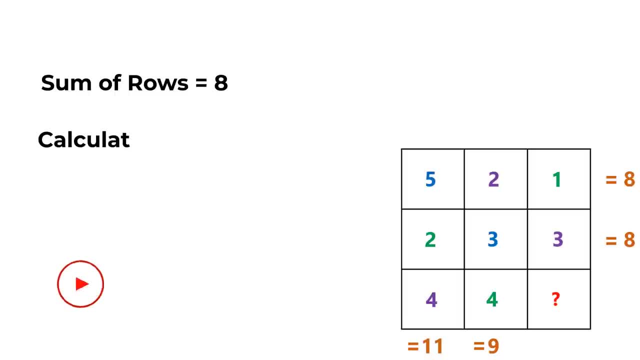 row. If we know that the sum should be 8, we can assume that the 4 plus 4 plus question mark, which would be representing the missing number, would be equal to 8.. So the missing number would be equal to 0.. The correct choice here is choice A, 0.. Hopefully you've nailed it. 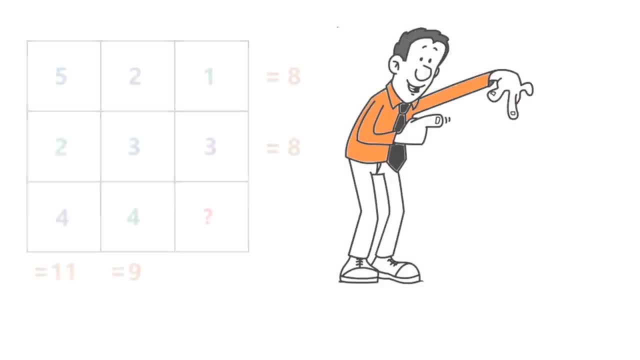 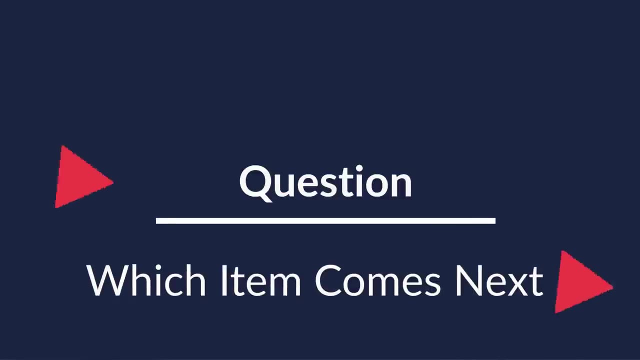 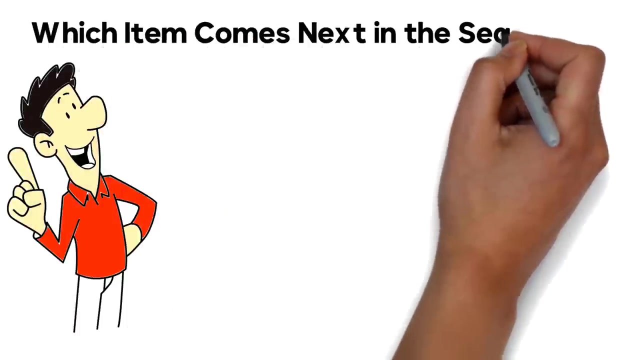 Take this question on your own and now know how to answer similar problems on the test. Very frequently on the test, you might be asked to detect the pattern. In this question. we're being asked which item comes next in the sequence And we're presented with the sequence. 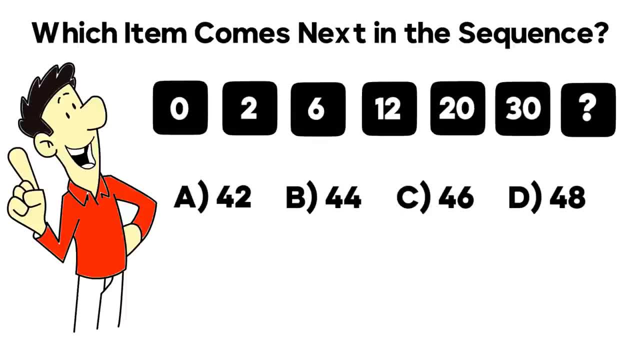 of items. Six items in the sequence are visible: 0,, 2,, 6,, 12,, 20, and 30.. And the next item is missing And you're being asked to select one of the four following choices: Choice A- 42.. Choice B- 44., Choice C- 46. And choice D- 48.. Do you see the 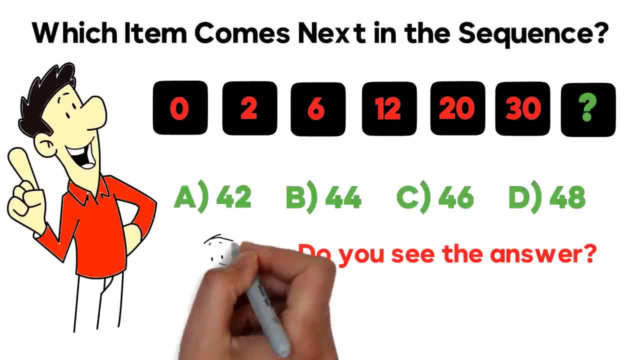 answer. It may or may not be obvious, depending upon your skills of detecting the pattern, Like it or not. we're going to continue and I'll share with you the answer in the next video. As with any type of question, the key is to determine the pattern, To determine the answer. 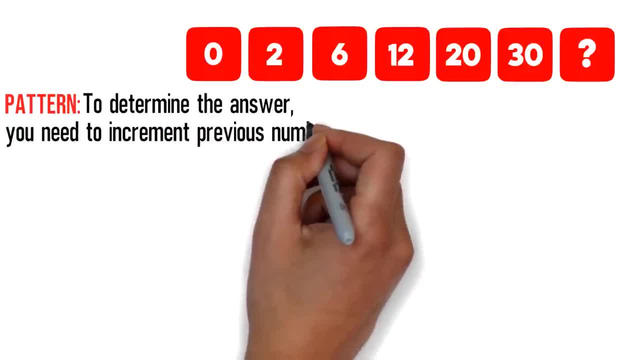 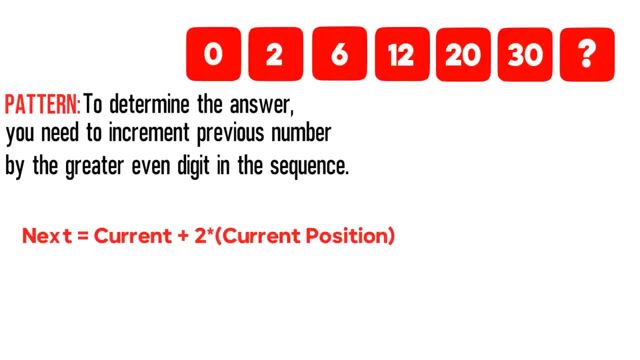 in this particular case, you need to increment previous number by the greater even digit in the sequence. You can even come up with the formula, And in our case, the formula to determine the next number would be current number plus 2 multiplied by current position. Let's see how it. 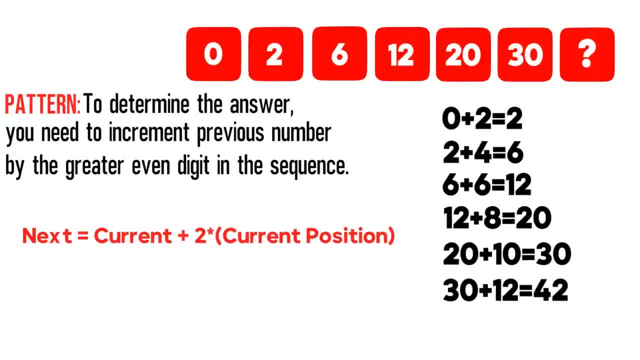 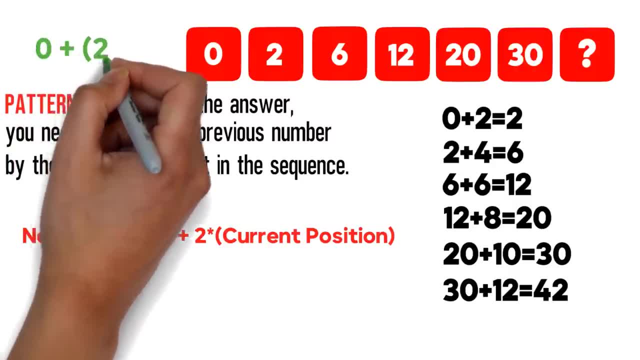 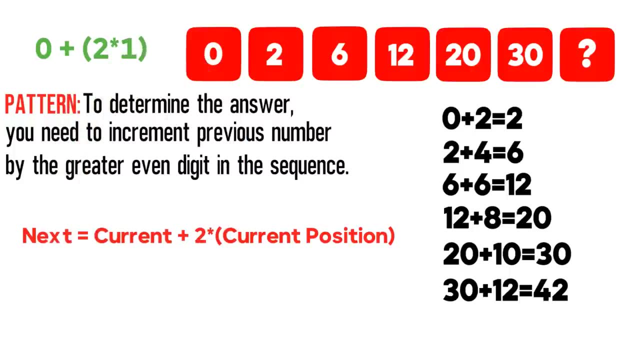 works. For example, let's take the number 0. This is the first number And in this case it's 0.. To determine the next number in the sequence, we need to add previous number, which is 0, and then 2 multiplied by 1.. Because number 0 has the first position in the sequence. 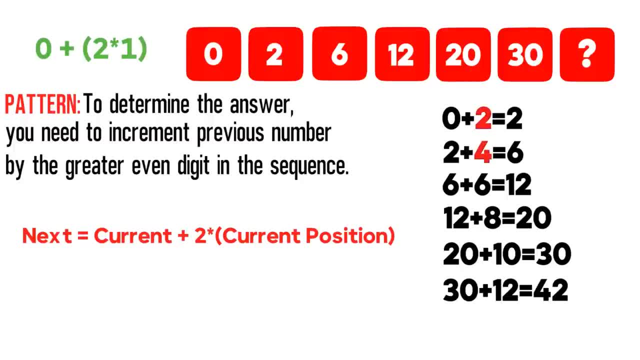 Instead of using the formula, you can also use the next even number and add it to the previous number. The even numbers are 2,, 4,, 6,, and you can increment them down the list, So you can add 2 to 0.. The next one would be 4.. And you can increment them down the list, So you can add. 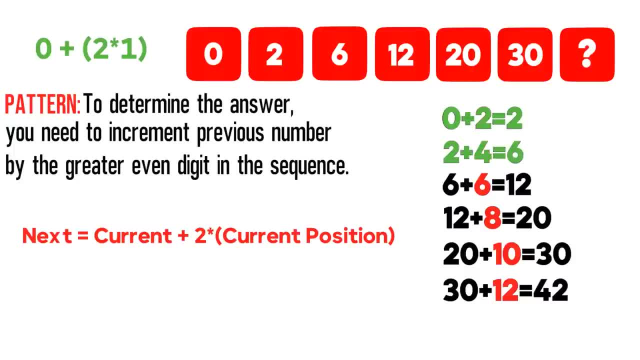 2 to 0.. The next number would be 6.. 6 plus 6 is 12.. The next number would be 8.. And 12 plus 8 equals 20.. The number after that would be 10.. So 20 plus 10 would be 30. And the number after that. 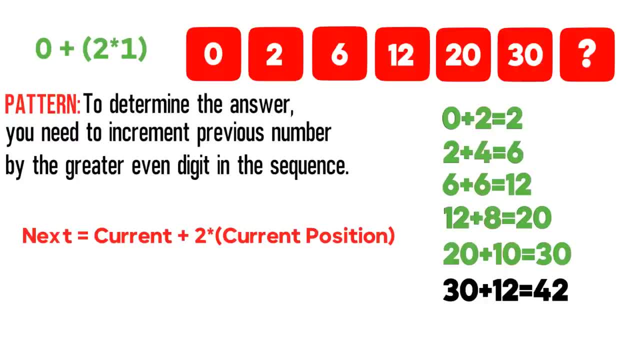 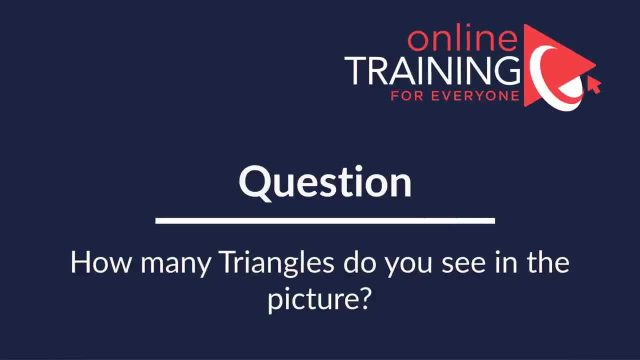 would be 12.. And 30 plus 12 equals 42. The correct choice here is choice A, 42.. Hopefully you've nailed this question and now know how to answer similar problems on the test. This is one of my favorite questions and there is a very high chance that you will get it on the 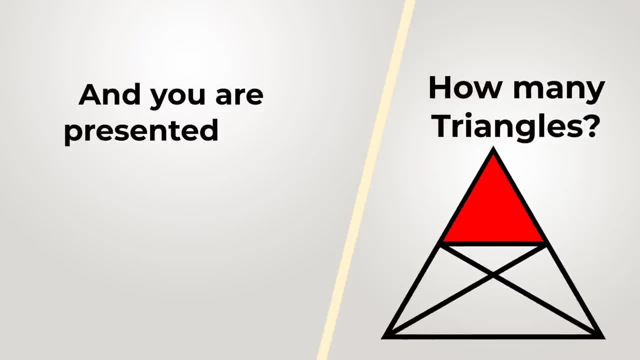 assessment test. How many triangles do you see? You're presented with the shape. on the left. There's a large triangle and there are also lines inside of this large triangle. You have four different choices: Choice A: 9 triangles. Choice B: 12. Choice C: 17. And. 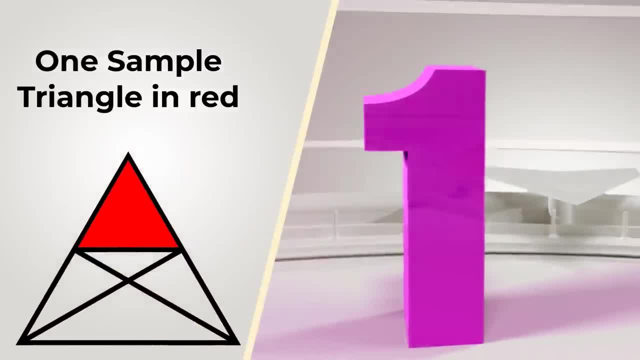 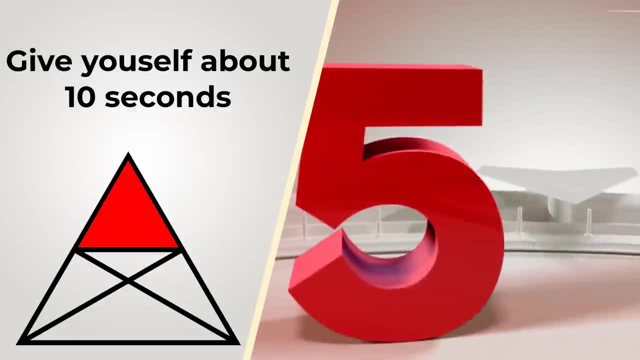 D 24.. One triangle is highlighted. It's highlighted in red, but there are a lot of other triangles. Do you think you know the answer? Give yourself a few seconds. I would recommend 10 to 15 seconds. This is about as much time as. 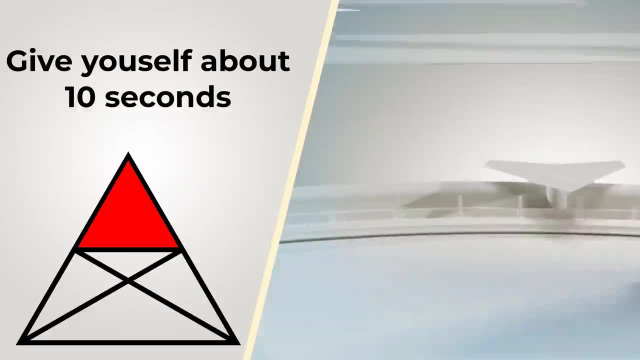 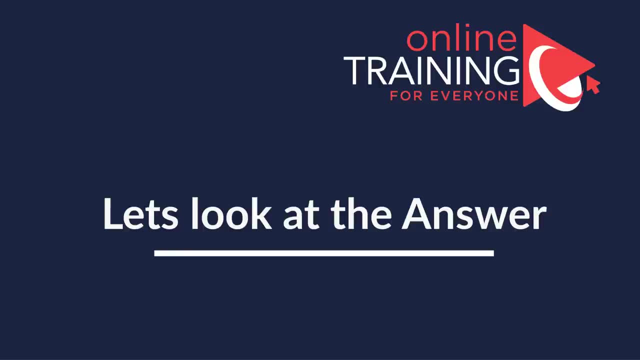 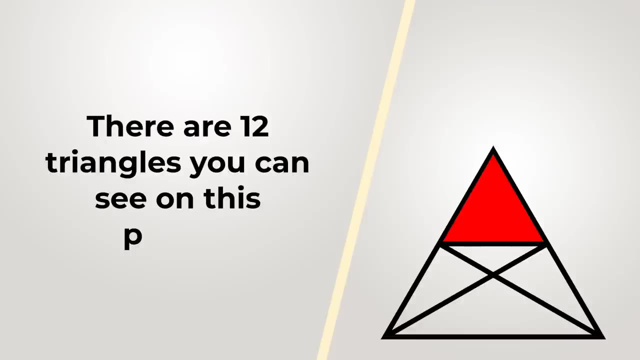 you will get in the real test. You can pause this video to give yourself some time to figure out the answer. I'm going to continue and reveal the correct solution so we can get to the answer together. I counted 12 triangles on this picture. Is this what you got too? Let me show them all, for. 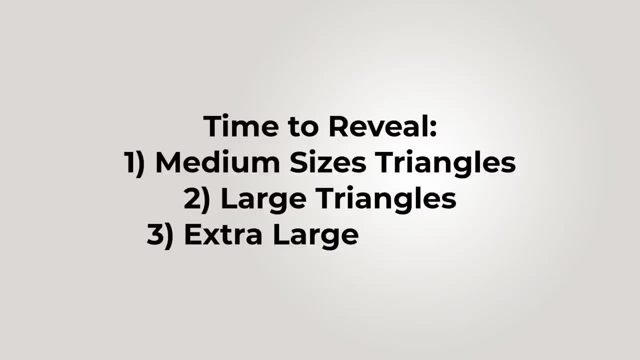 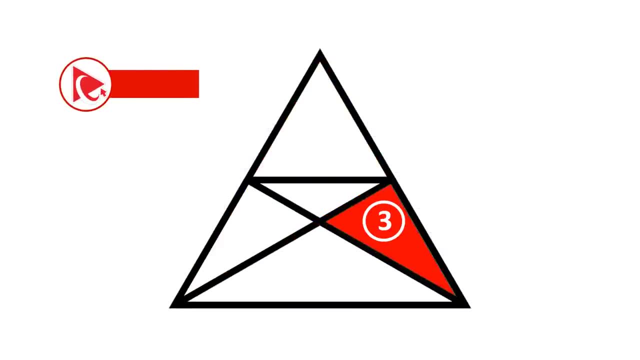 you. I'll start with the smaller triangles and then go to the medium-sized ones and then go to the large ones: 1,, 2,, 3,, 4,, 5,, 6,, 7,, 8,, 9,, 10,, 11, and 12.. 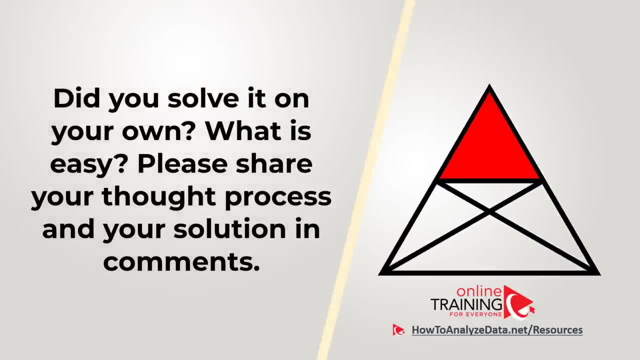 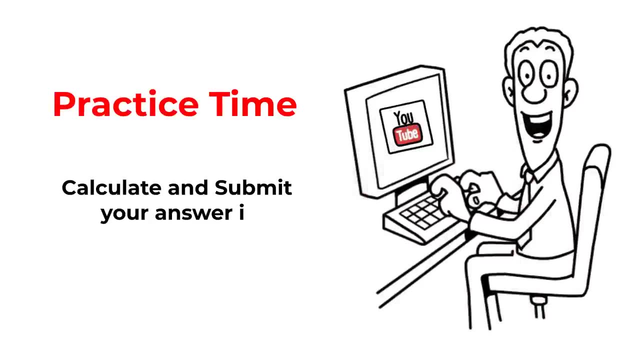 Did you come up with the different answer? Please share your thought process in the comment section of this video so we can all learn from your perspective. Hopefully you nailed this question and got to the correct answer on your own. And now here's the question for you to try. If you can calculate the answer, please post it. 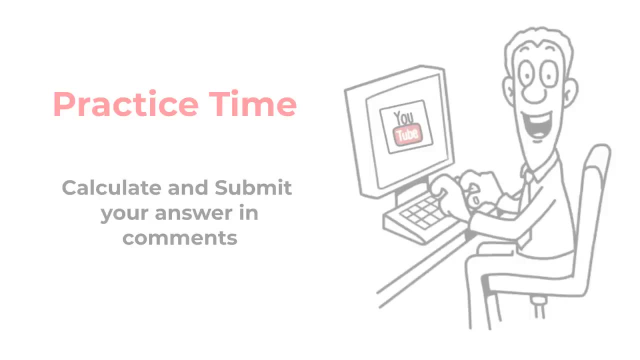 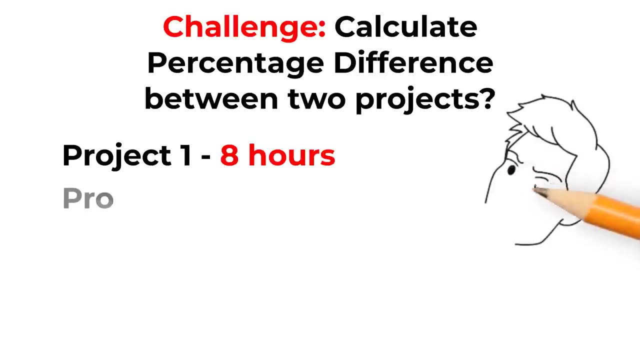 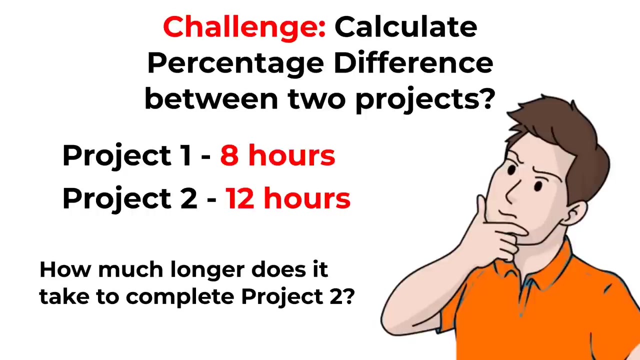 in the comment section of this video so I can give you the grade. We have two projects and to complete project 1, it takes 8 hours and to complete project 2, it takes 12 hours. So how much longer in percentages it takes to complete project 1 versus project 2?? 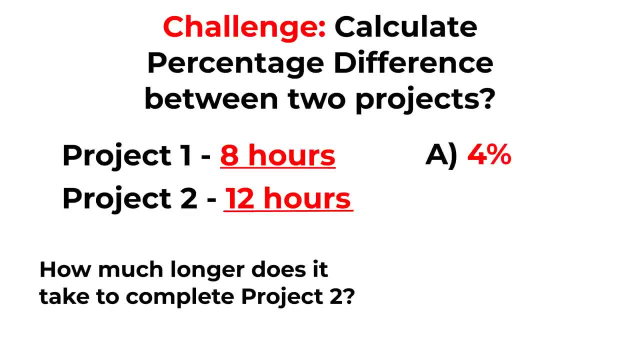 You have four different choices: Choice A – 4%, choice B – 50%, choice C – 100% and choice D – 150%. Can you calculate the answer? Please make sure to post it in the comment section of this video so I can give you the grade. Thanks for participating and good luck. 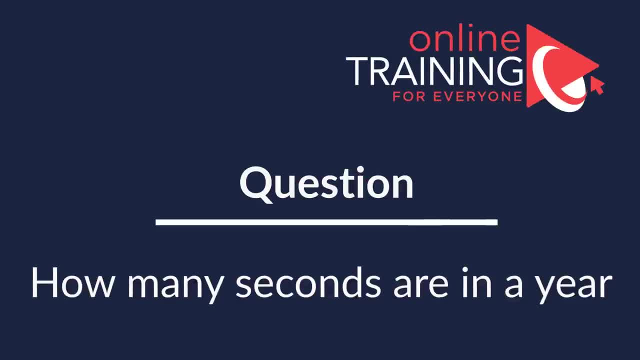 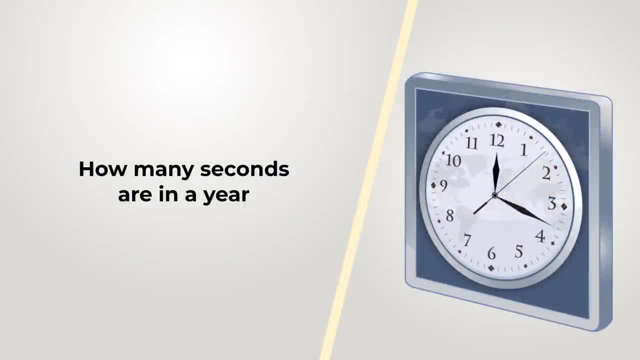 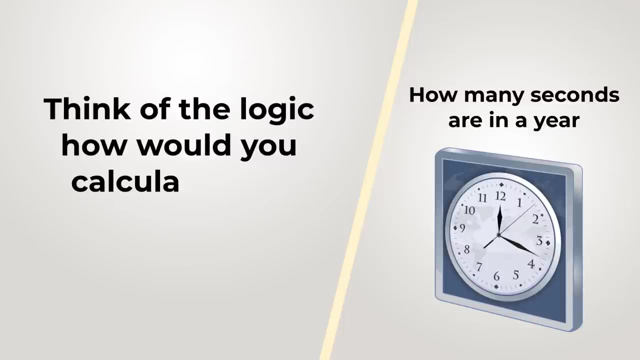 I had this question being asked as part of consulting job interview. How many seconds are there in a year? Take a look at the picture. It might give you a hint. Do you think you know the answer? Think of the logic. how would you calculate how many seconds are there in? 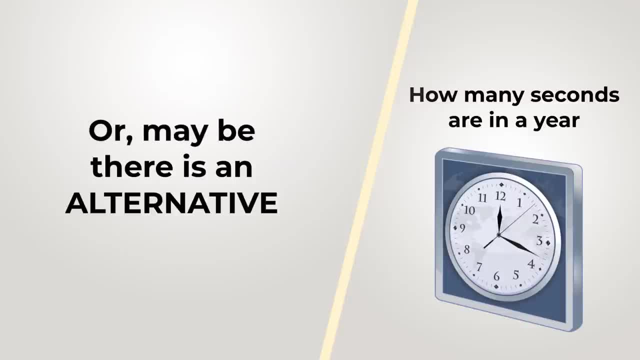 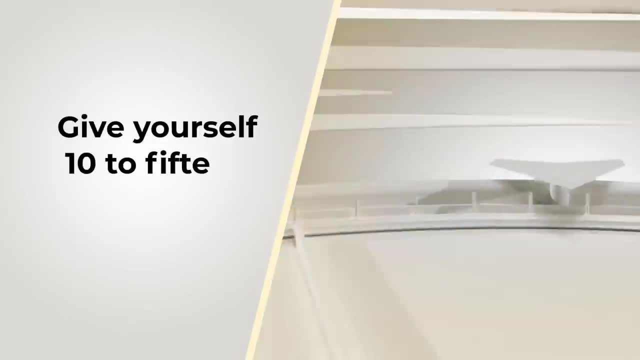 a year, Or maybe there is an alternative. Always try to think out of the box- This would be my hint to you- And give yourself 10 to 15 seconds. This is as much time as you might get answering these types of questions in the test. 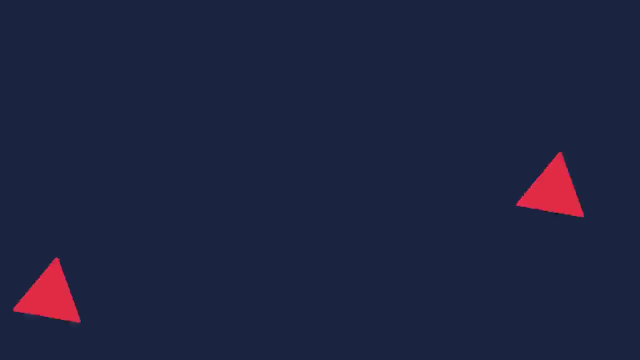 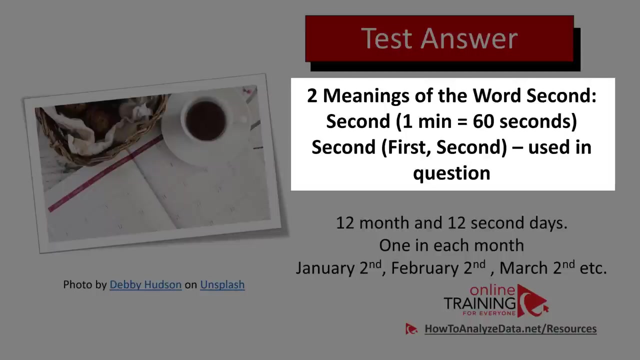 Now let's continue and get to the correct solution together. Obviously, this is a tricky question and challenges you in understanding of the word second. There are two meanings in the word second. One is second. For example, one minute has 60 seconds, But second. one is second, where you have sequence of first and second. 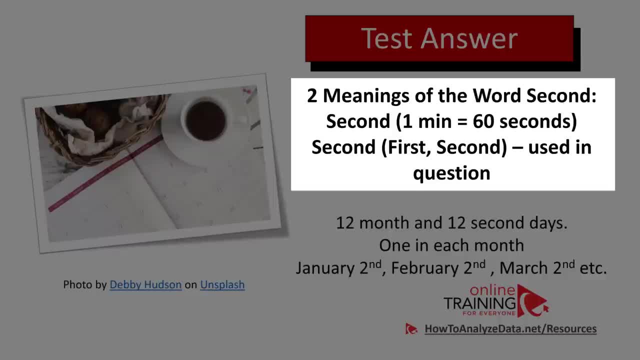 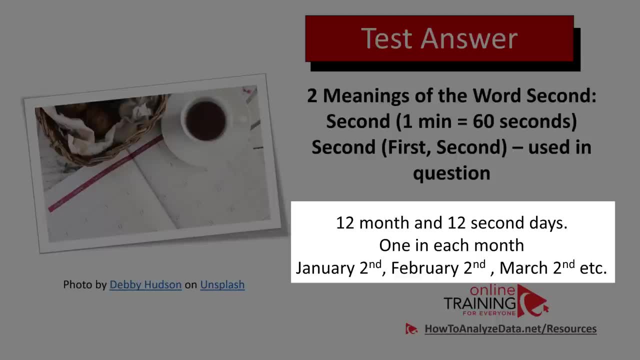 And the second meaning of the second is used in this particular question. so, if we go back to the question, in the year there are 12 months and there are 12 second days. one second day in each month: january 2nd, february 2nd, march 2nd. 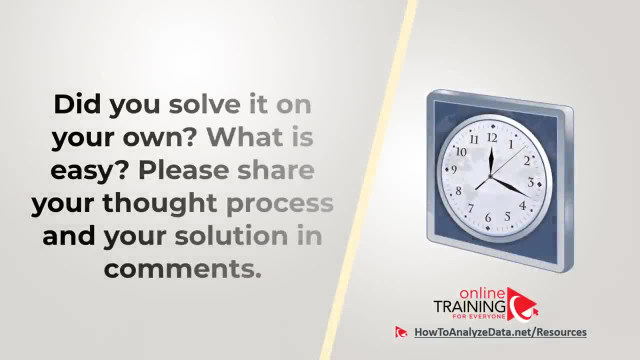 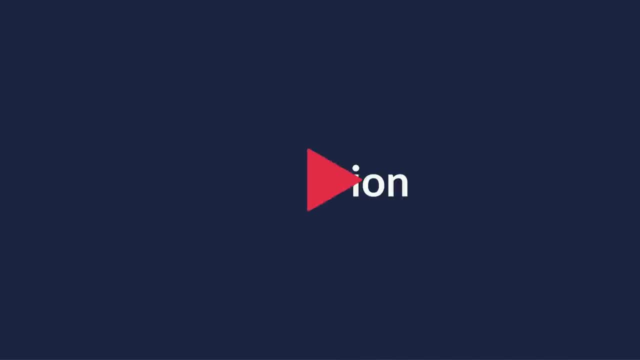 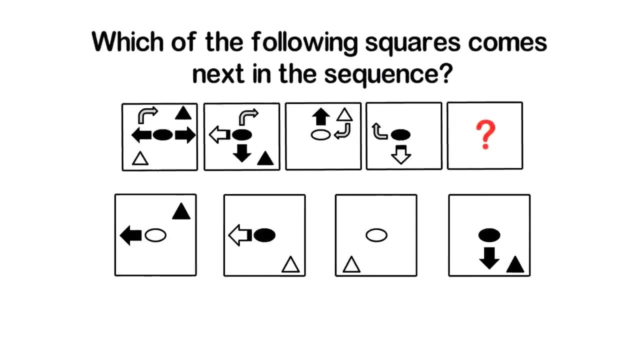 and etc. hopefully you've nailed this question. it gives you some laugh and you now know how to answer similar problems on the test. here's the question that on the surface seems very, very hard to solve, but in reality, the answer to this question is very simple: you're. 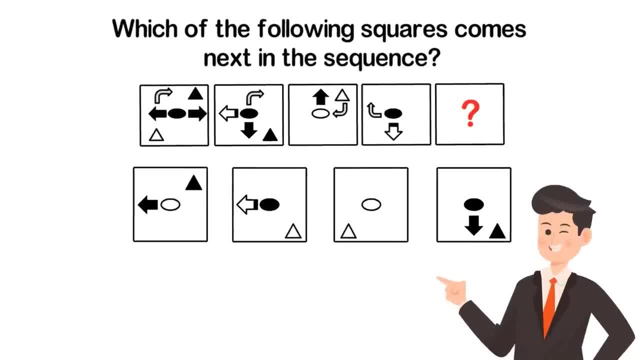 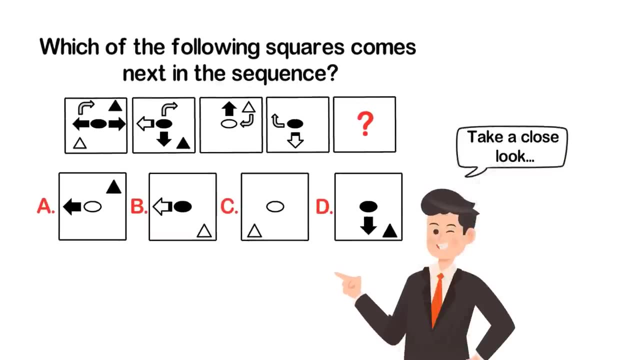 presented with five different squares. squares one through four have shapes inside and you need to determine the missing square five. you're presented with four different choices: a, b, c and d. take a close look to see if you can come up with the correct answer- maybe give yourself. 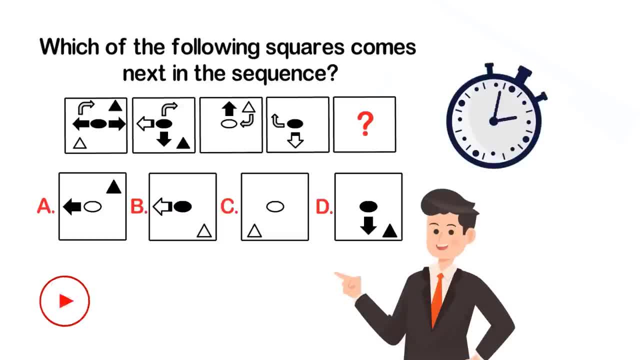 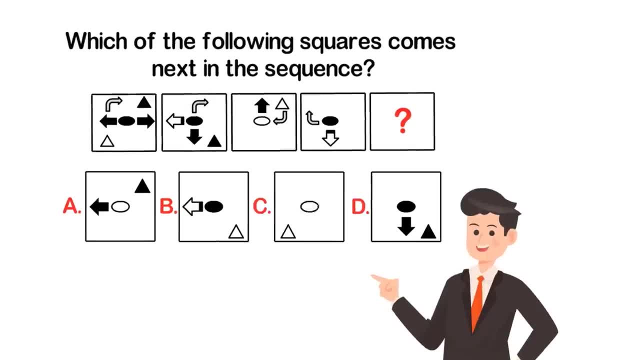 five to ten seconds, or maybe longer- 10 to 20 seconds. this is about as much time as you'll get on the real test. did you figure out the answer? let's continue to see how we can solve this challenge and get to the correct solution together. as i mentioned, test writers are trying to trick. 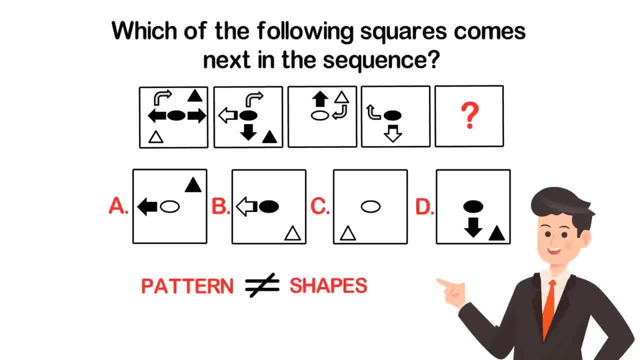 you and in this particular case, there is no pattern within the shape. it's all random. no matter how hard you try, you will not be able to determine the missing square five or more of the three of them in the test form. you will definitely be able to fix it, but you will never be able to solve the problem of the right question. 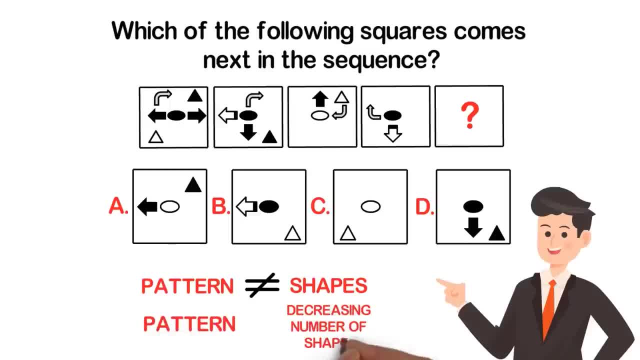 any patterns among those small shapes. the pattern here is the decreasing number of shapes. if you look at the figure one, it has six shapes. if you look at the figure two, it has five, four, three. so the answer for the figure five: the number of inside shapes should be two. so the correct answer. 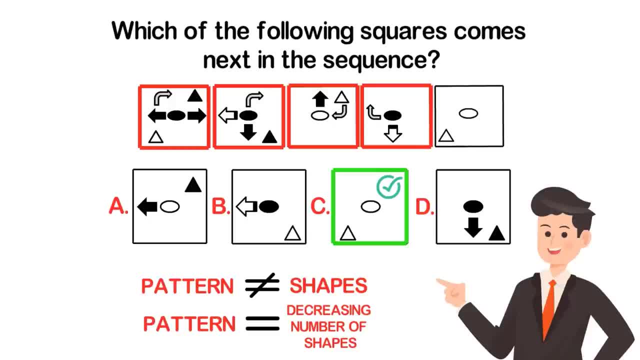 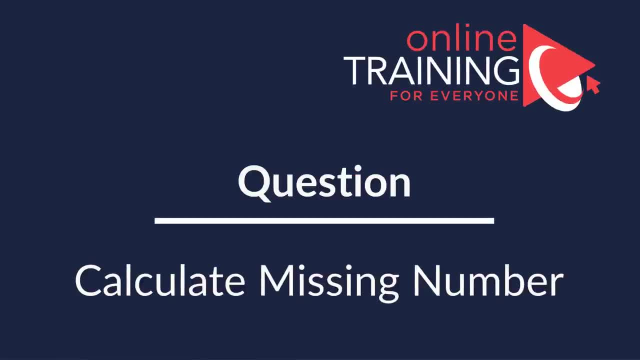 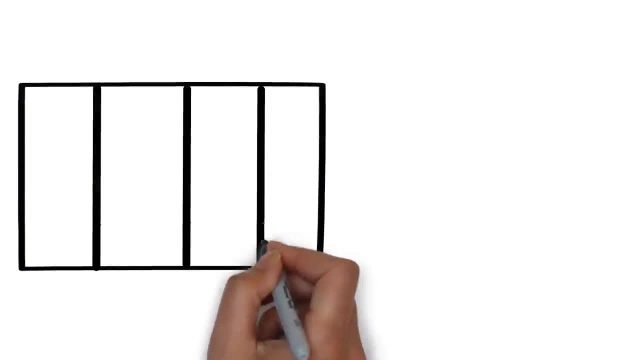 here is choice c. hopefully you nailed this question and now know how to answer similar problems on the test. here's one of my favorite questions because it is very frequently used in the test. you're presented with the matrix four by three matrix. each cell in the matrix has numbers. 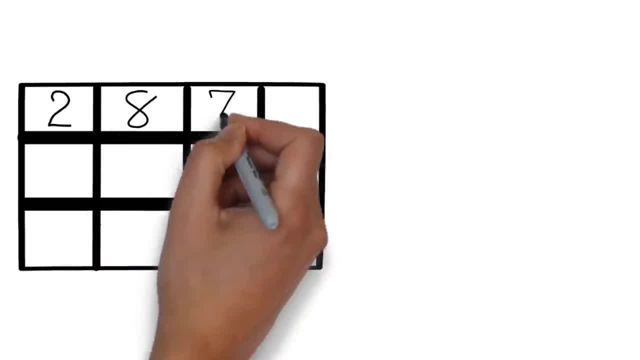 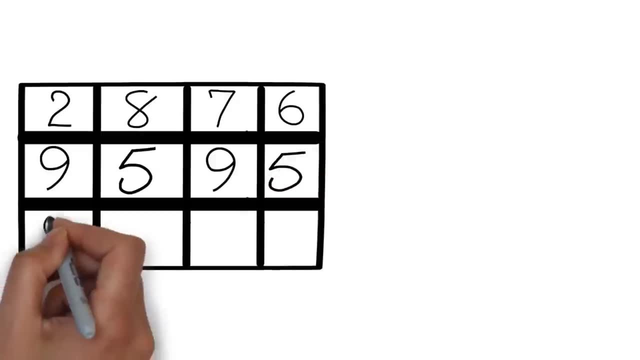 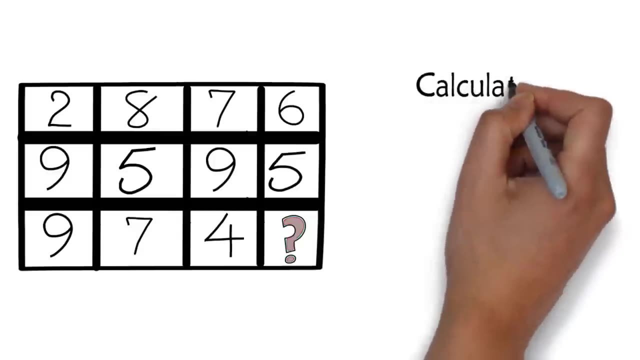 for example, first row in the matrix has numbers two, eight, seven and six. second row has numbers nine five, nine five and the third row has numbers nine, seven, four and one number in the bottom right corner is missing, and this is exactly what you need to calculate. you can choose from one of four different choices: choice a- 5, choice b- 7. choice c- 9. 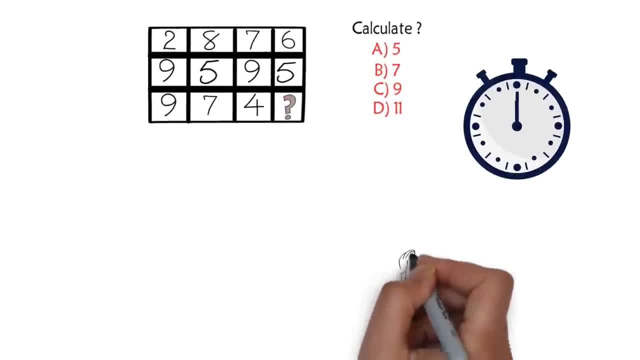 and then choice d 11.. do you think you can come up with the answer? give yourself 5 to 10 seconds. this is about as much time as you will get on the test. let's continue to see how we can get to the correct answer together. 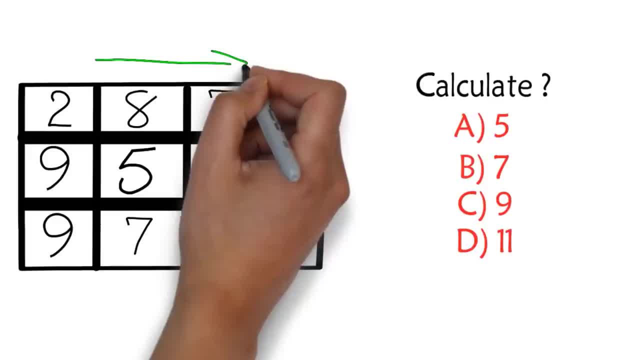 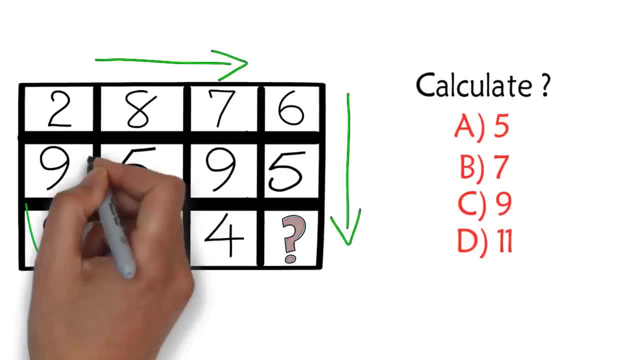 the key to solve this problem is to determine the pattern, and the pattern either can be in the rows or in columns. in this particular case, let's check the columns first, and then what you see is that each column adds up to the value of 20.. for example, 2 plus 9 plus 9 is 20.. 8 plus 5 plus 7 is 20.. 7 plus 9 plus 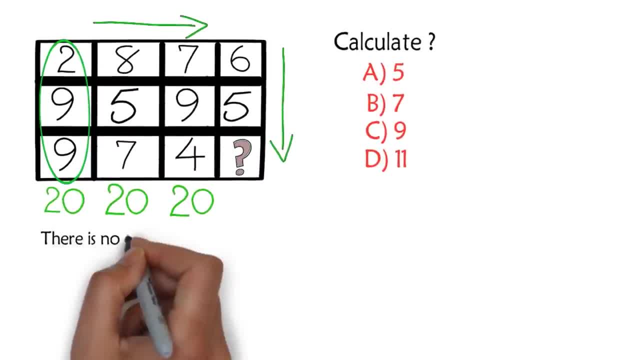 4 is 20 as well. we also want to check if there is a pattern with the rows. and there is no pattern, because the first row adds up to 23.. 2 plus 8 plus 7 plus 6 equals 23, and the second row adds up to 28: 9 plus 5 plus 9. 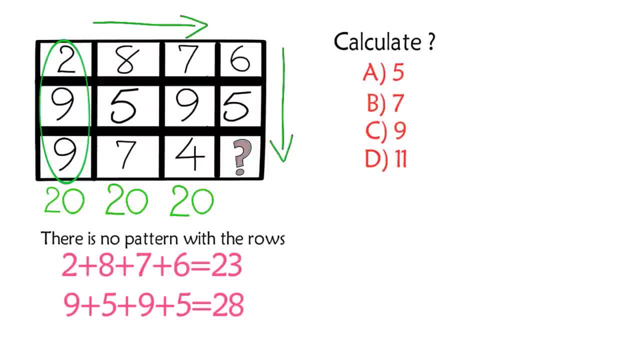 plus 5 equals 28, so there is no pattern. based on this information, you can calculate the missing value in the fourth column: 6 plus 5 plus question mark equals 20.. so the answer is c 9. this is the missing value. hopefully you figured it out and now know how to answer. 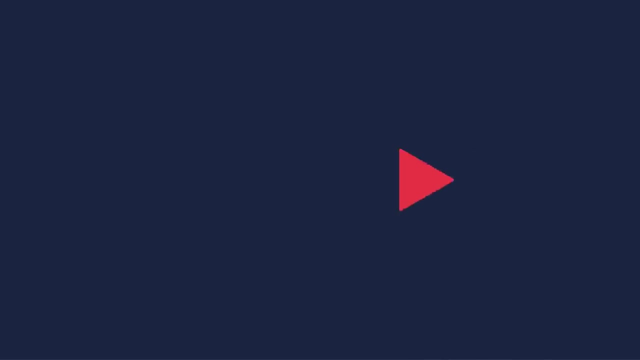 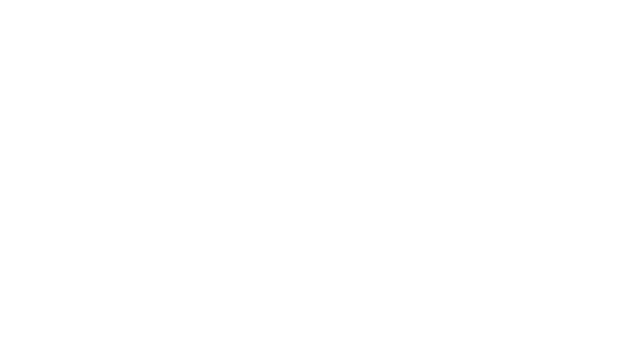 similar problems on the test. Here is another puzzling question you might find difficult to solve. You are presented with four triangles. Each triangle has a number in the corner and you need to calculate one of the missing numbers in the upper corner of the black triangle. You have four. 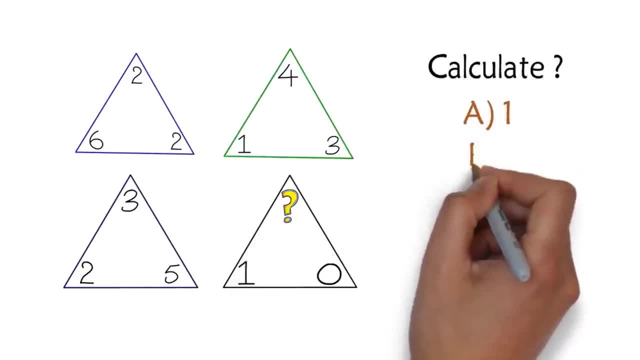 different choices. You have choice A, 1.. You have choice B, 2.. You have choice C, 3. And you have choice D, 4.. Can you determine the answer? Let's continue to see how we can solve this challenge. 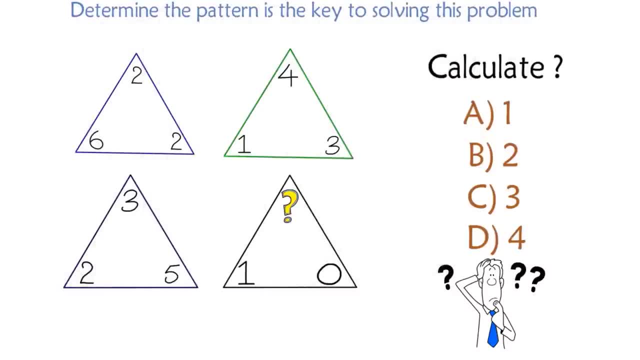 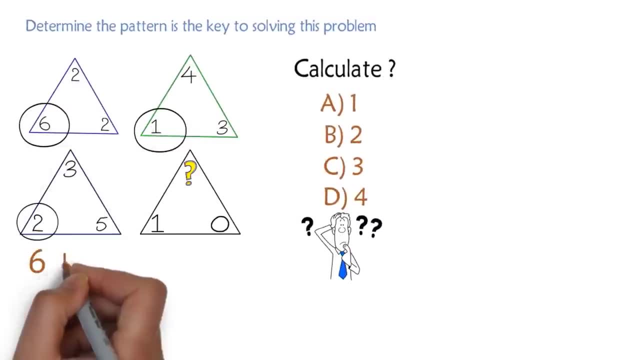 together. Determining the pattern is the key to solving this challenge. For example, if you add up the numbers in the lower left corners, 6 plus 1 plus 1 plus 2 in all triangles, you will get to the solution. You will get to the solution. You will get to the solution. You will get to the 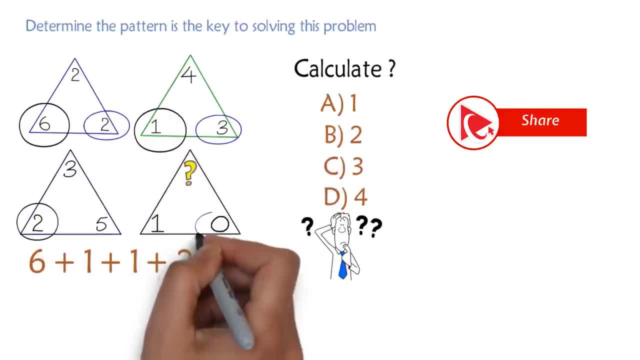 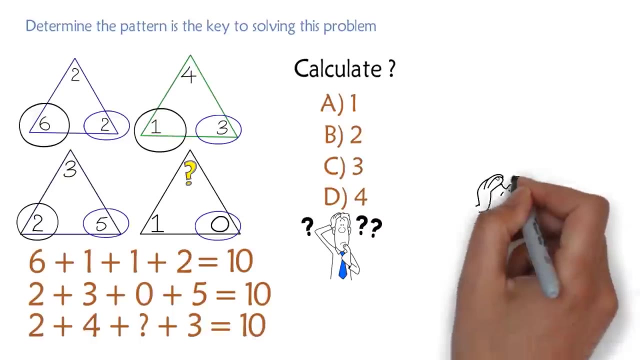 10.. Same thing happens when you add up the numbers in the bottom right corners of the same triangles: 2 plus 3 plus 0 plus 5 also equals 10.. So same logic can be applied to the upper right corners of the triangles. As you can see, triangles are colored to confuse you, So you're only. 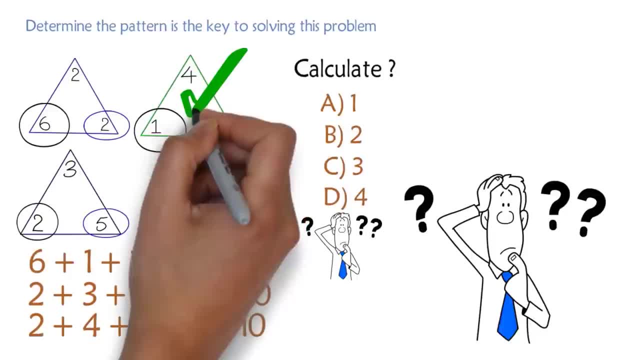 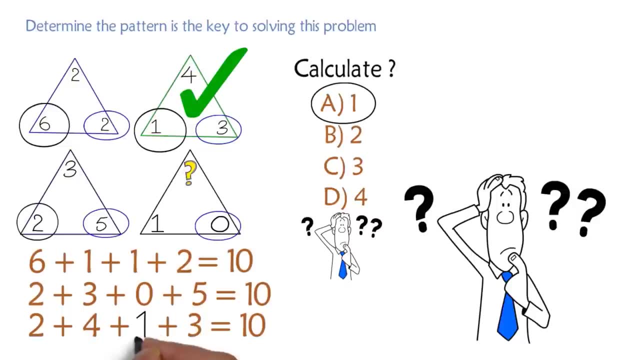 concentrated on the numbers inside of each triangles, but you're not looking across multiple triangles. The correct answer to this problem is choice A, 1. Because this is the math of getting into 10 with the missing number. Hopefully you've nailed this question and now know how to answer similar problems on the test. 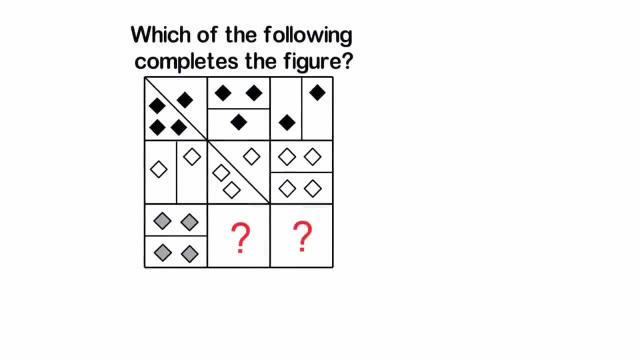 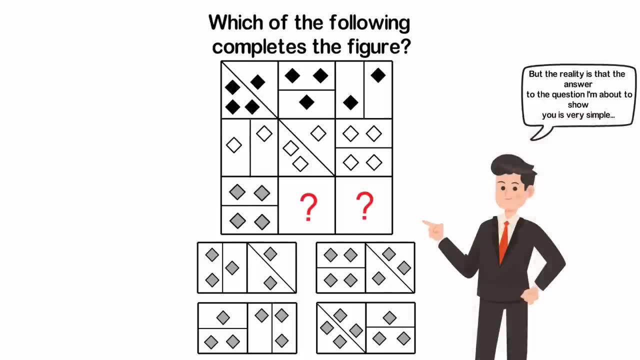 When you see a question like this, you might ask yourself how can it possibly be even more confusing? But the reality is that the answer to the question I'm about to show you is very simple. Let's look in more details. You're presented with the 3x3 matrix. 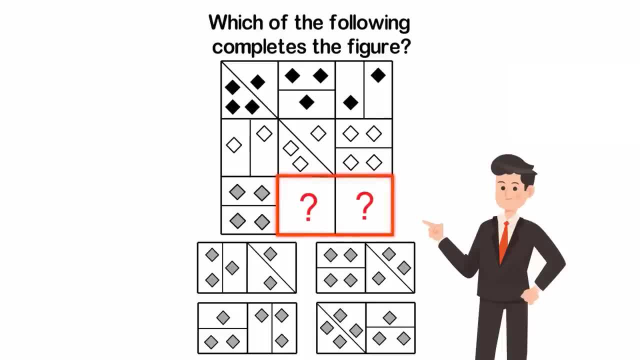 The shapes in the matrix are missing. They are located in the bottom row And you have 4 possible choices for the answers: Choices A, B, C and D. Take a close look. The solution is not obvious, but it is very simple. Give yourself 10-20 seconds, maybe go to 30 seconds. 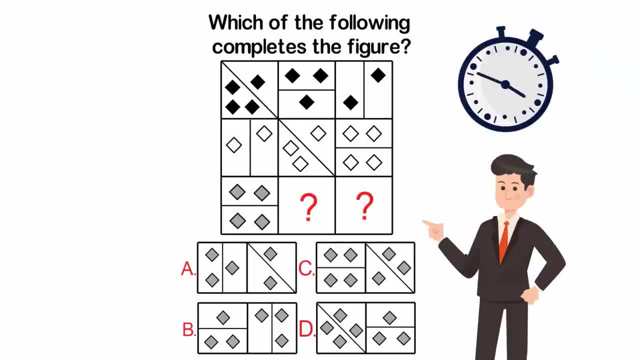 by pausing this video to see if you can come up with the answer on your own. Are you ready? Let's continue to see how we can get to the correct solution together. As I mentioned, the answer to this question is very simple. The pattern is represented in each row by decreasing. 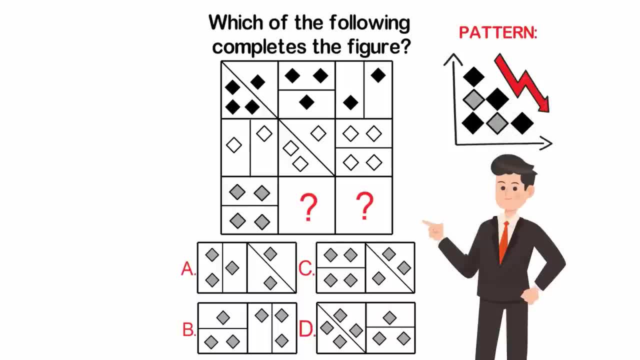 number of diamonds. Let's look at the top row. You see that the top left square contains 4 black diamonds. The middle square in the top row contains only 3 diamonds, And then the right square in the top row contains only 2 diamonds. In the second row the pattern reverses and it. 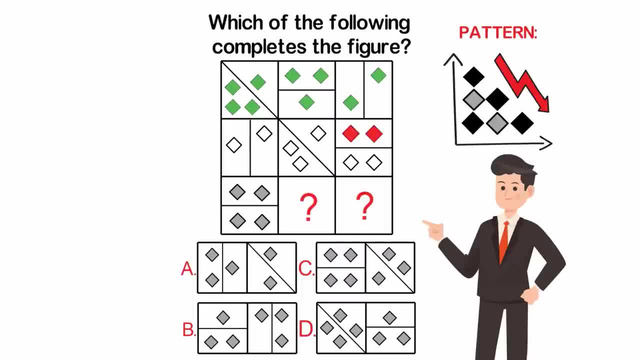 goes from right to left And you see the same pattern of the white diamonds: 4 goes down to 3 and then goes down to 2.. So in the bottom row we need to follow the same pattern. The pattern will be the number. 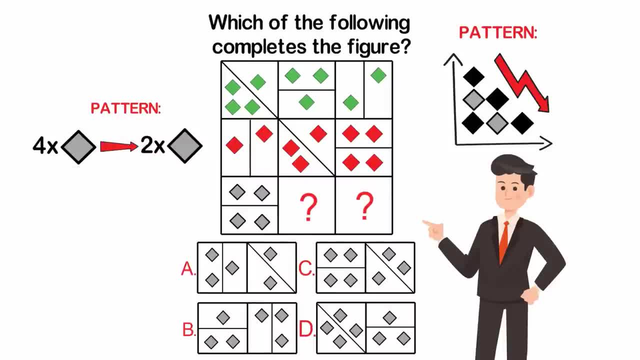 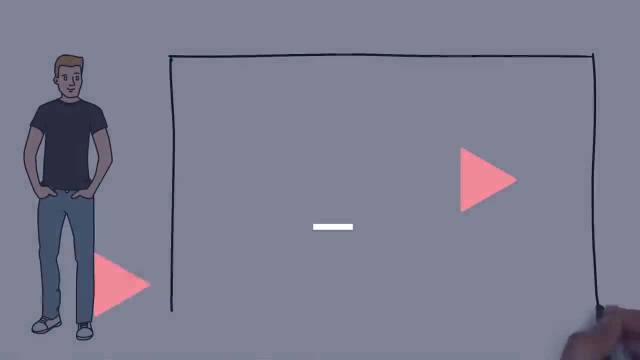 of diamonds, decreasing from 4 to 2 among the gray diamonds. So the correct answer here is choice A. Hopefully you've nailed this question and now know how to answer similar problems in the test. This is one of my favorite questions because it is very frequently used in the test. You 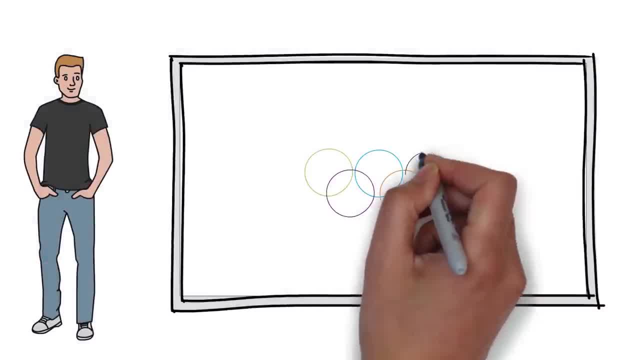 are presented with 5 crossing circles. All circles are of the different colors. There are numbers inside the circles. The number of diamonds is the number of diamonds. The number of diamonds is the number of circles. The number of diamonds is the number of circles. 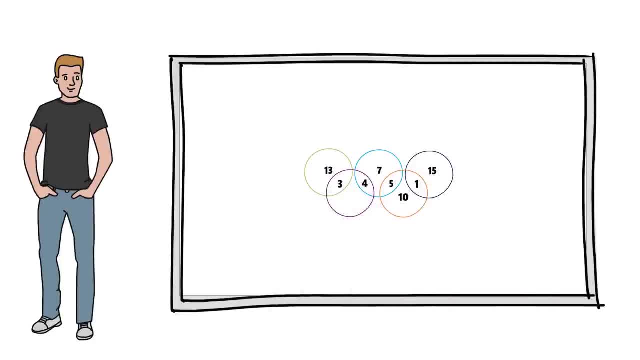 And the number of diamonds is also the number of circles. If I am going to measure the number of diamonds in the test, I should substitute the numbers of diamonds on the intersections of the circles. In this particular case, you are presented with five different circles, all of them different colors, and the numbers that you see on the 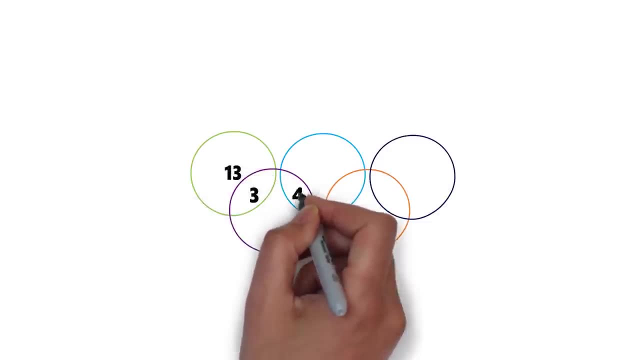 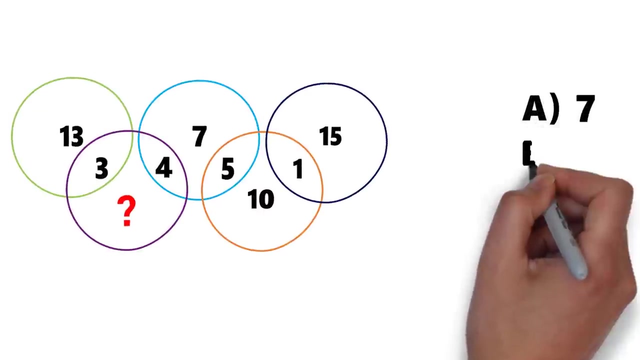 screen are 13,, 3,, 4,, 7,, 5,, 10,, 1, and 15.. There is also one number missing which is highlighted with the question mark. You need to calculate the missing number and the choices are Choice A – 7, Choice. 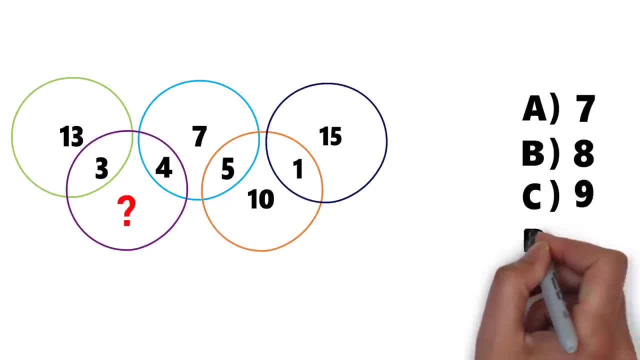 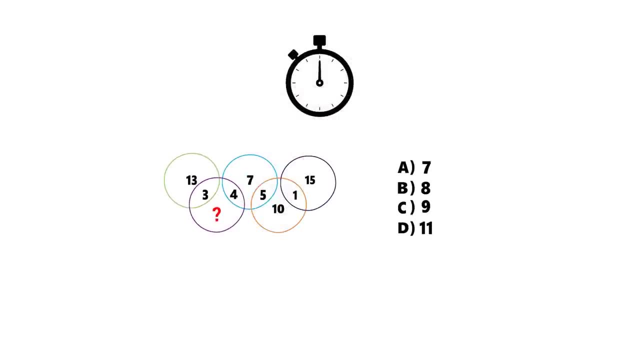 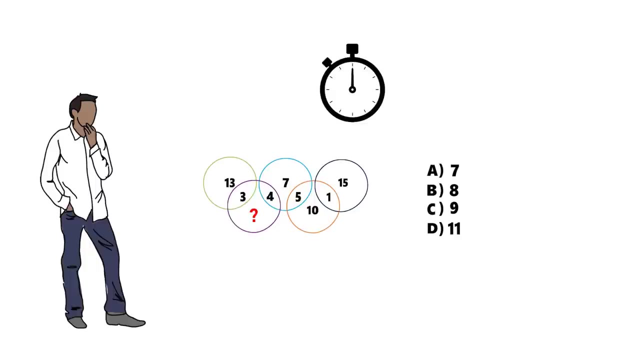 B – 8. choice c: 9 and choice d: 11. give yourself few seconds, maybe 10 to 15 seconds. this is about as much time as you get on the typical test to calculate the answer. do you see the solution? let's continue to see how we can get to the correct solution and solve this challenge together. 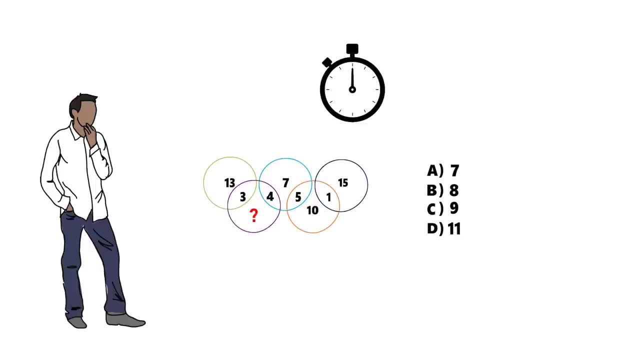 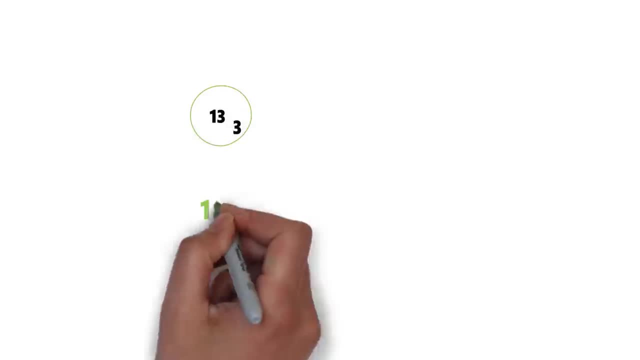 as you might have figured out by now, sum of each numbers in the circle adds up to 16.. for example, let's look at the green circle. we have numbers 13 and 3, and 13 plus 3 equals 16.. in the blue circle, 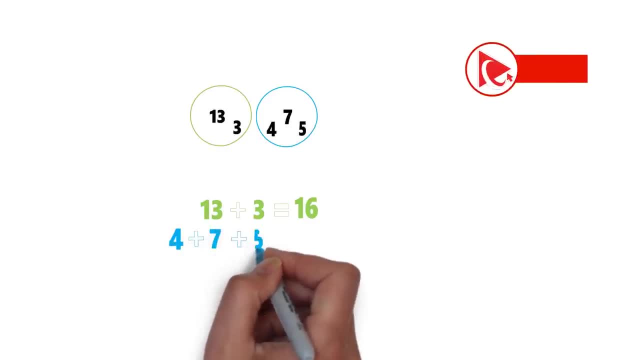 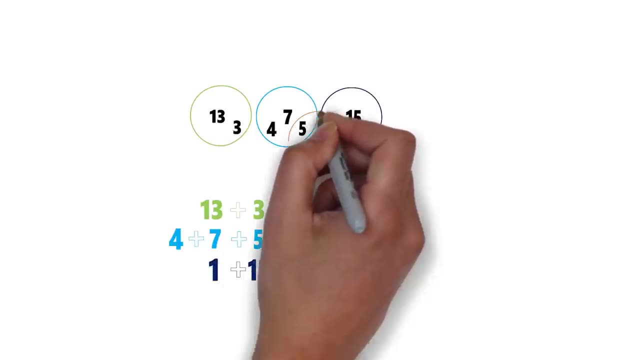 we have numbers 4 plus 7 plus 5, and all of them add up to 16.. in the black circle we have 1, and 15 also adds up to 16, and in the orange circle we have 5 plus 1 plus 10 also equals 16.. so to: 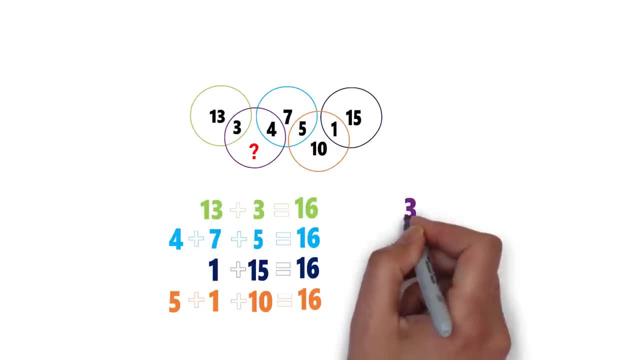 calculate question mark, which is the missing number, we need to add 3 plus 4 plus question mark. so to calculate question mark we need to add 3 plus 4 plus question mark and make an equation to make it equal 16.. after doing the calculation you see that the question 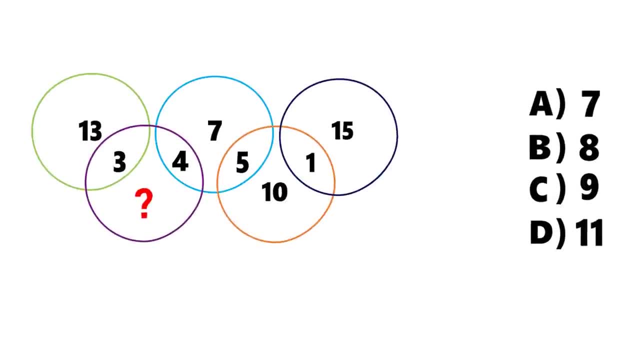 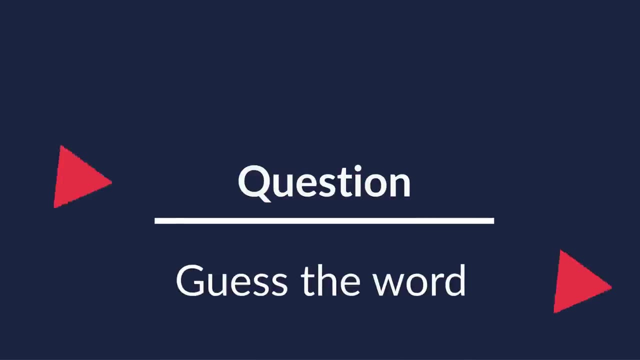 mark and the missing number equals 9.. so the correct choice here is choice c 9.. hopefully you've nailed this question and now know how to answer similar problems on the test. a lot of times you might be presented with the question in the test. that will try to. 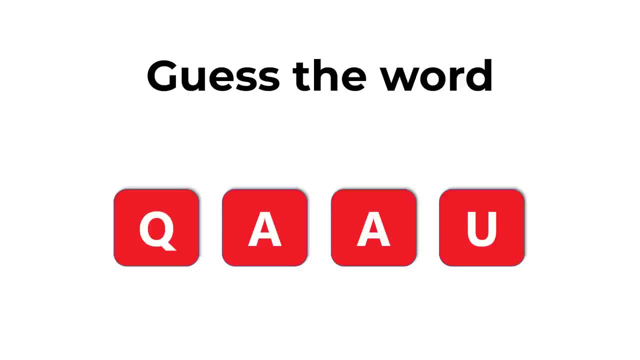 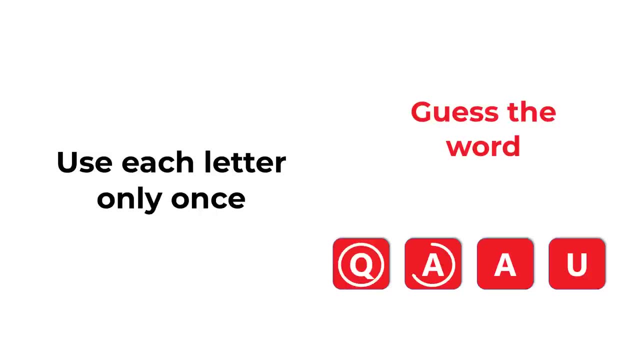 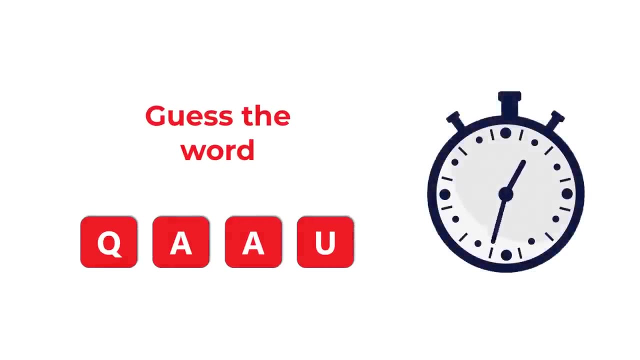 determine your knowledge of english words, as well as how quickly you can extract this words from your memory. in this particular case, we are looking at four letters- q, a, a and u- and you need to guess the word by combining these letters. do you see the word? give yourself five to ten. 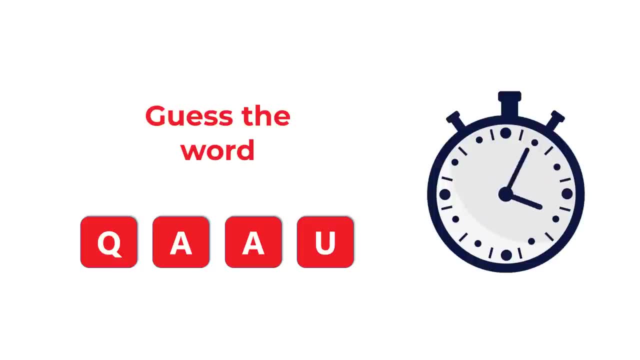 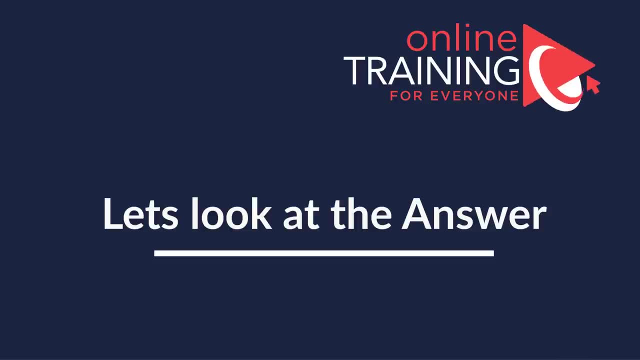 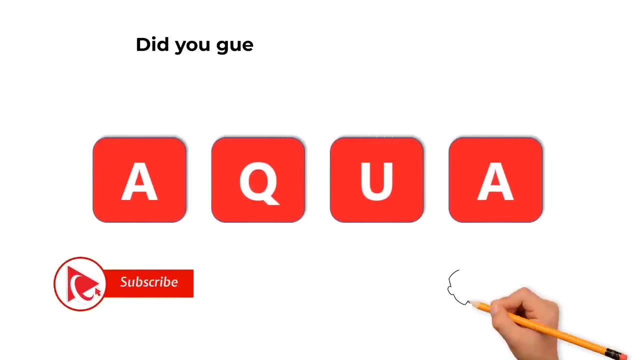 seconds to see if you can come up with the answer. let's continue to see how we can get the correct answer together. as you might have figured out, the correct answer here is word aqua. the spelling of the final word is a, q, u, a, and you can get to the correct answer by rearranging the letters on the 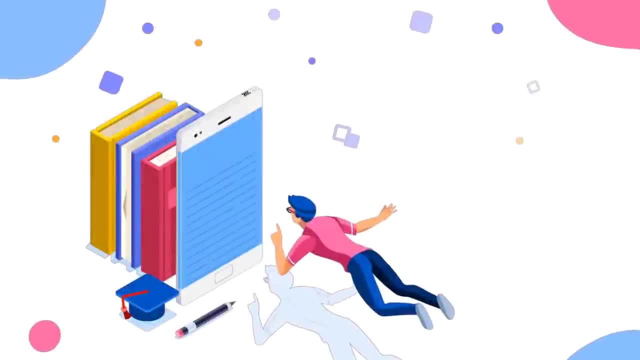 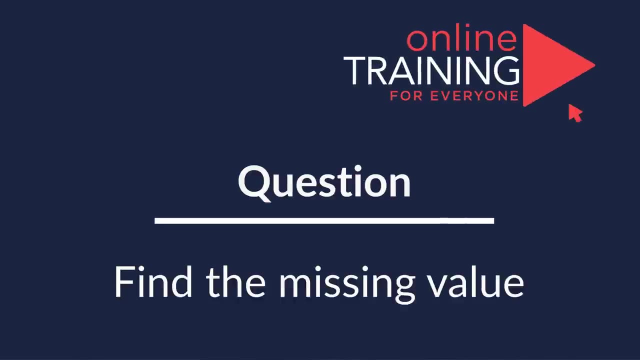 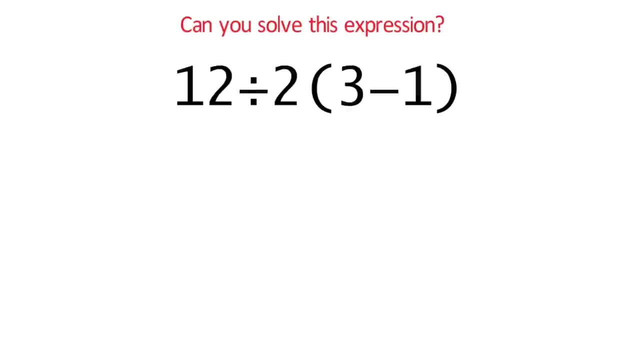 screen. hopefully, you've nailed this question and now know how to answer similar problems on the test. here's the interesting question, which is easy to understand but at the same time, you will have a lot of fun solving it. you need to calculate the simple expression 12 divided by 2 and then multiplied on the value in parentheses. 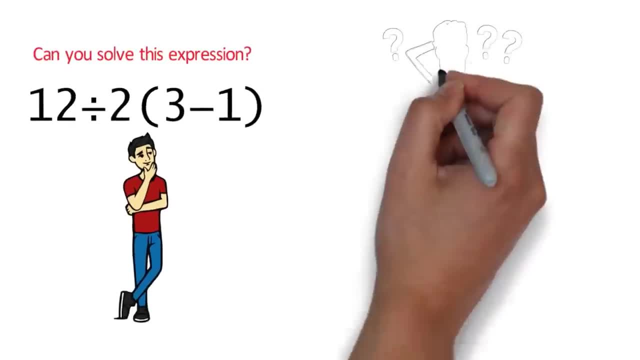 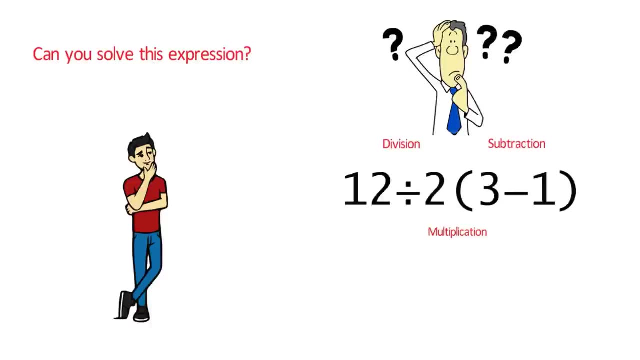 which is 3 minus 1.. take a look closely and see if you can come up with the answer. there are three operations here: division, multiplication and subtraction. all you need to determine is which one to do: first, second and third. do you think you know the answer? 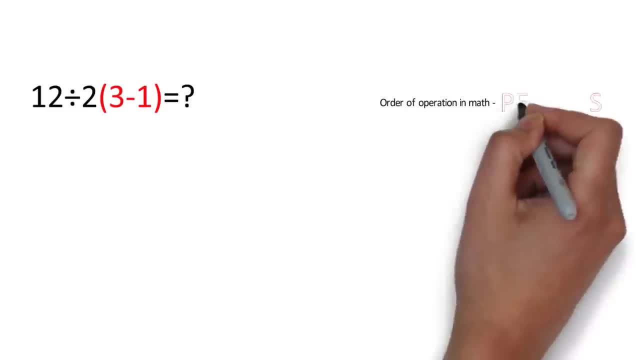 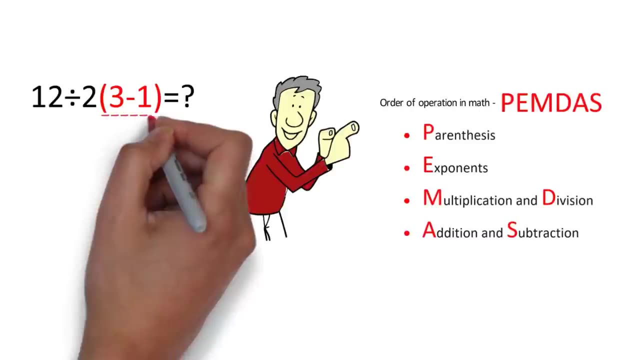 let's continue and get it solved together. the order of operations in math tells us that the first expression we need to solve is in parentheses. we first need to calculate 3 minus 1 and obviously the answer is 2.. the big question is: what do we do next? 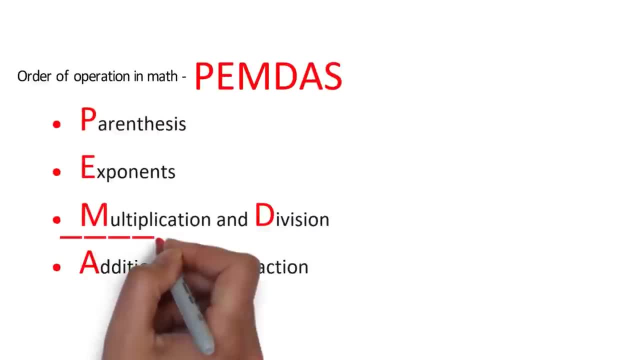 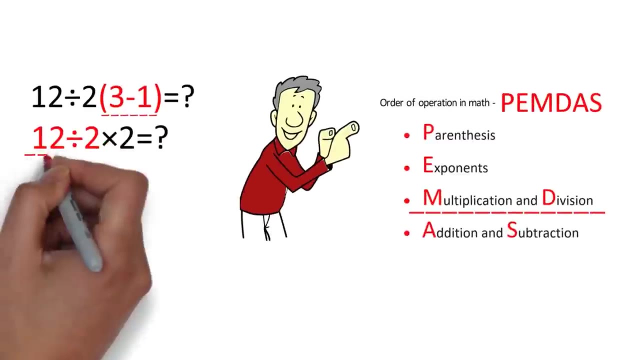 the order. pemdas tells us that we need to do multiplication and division, but what order doesn't mention is that we need to do it from left to right. and, what's interesting, the acronym itself is a little bit confusing because it shows multiplication first and then division. but in our case we need to do division first and divide 12 by 2 and then do multiplication. 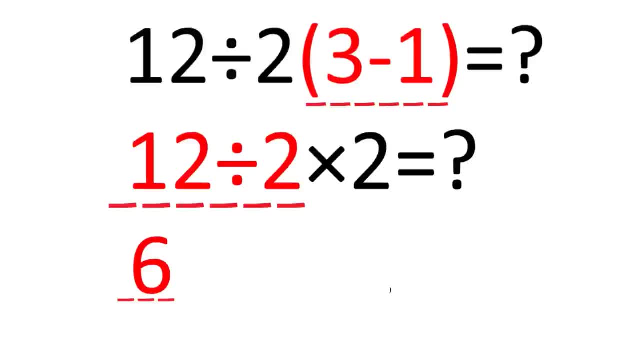 so let's first divide 8 by 6- we get 7 divided by 2, and then divide 12 by 2, and the final expression we need to solve would be 6 multiplied by 2, so the correct answer here is 12.. so did you solve this challenge on your own? 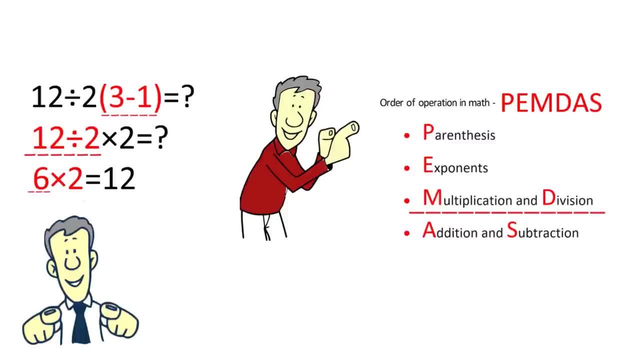 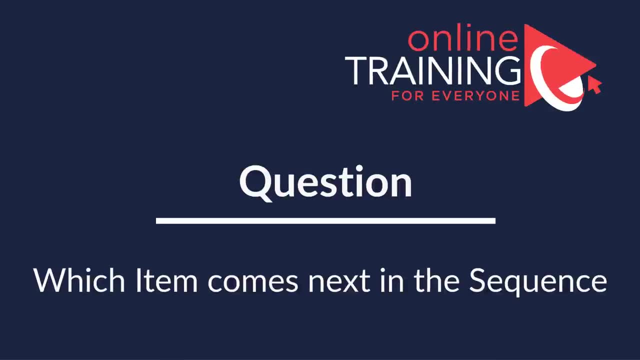 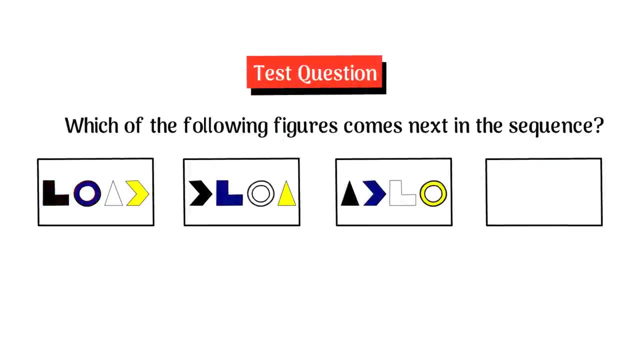 was it easy for you. please share your thought process and your solution in the comment section of this video. here is a very cool question that you frequently see on the test you're presented. In each one of these rectangles there are different shapes. Each shape is of the different color. 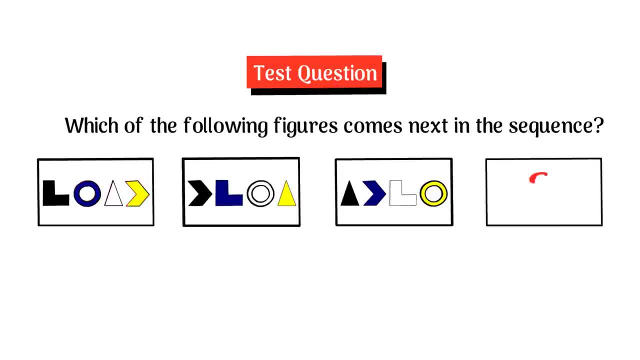 Three rectangles have shapes present and fourth rectangle on the right has all the shapes missing. You have four different choices to identify the missing item in the sequence: Choices A, B, C and D. Do you think you can come up with the answer? 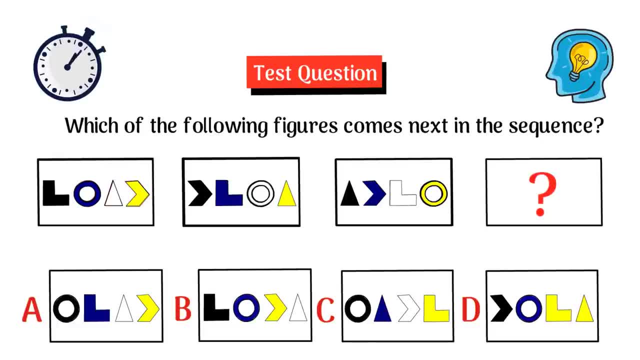 Give yourself some time. You can pause this video to see if you can identify the pattern. Give yourself 5 to 10, maybe 10 to 15 seconds. This is about as much time as you will get in a real test. Did you figure out the solution? 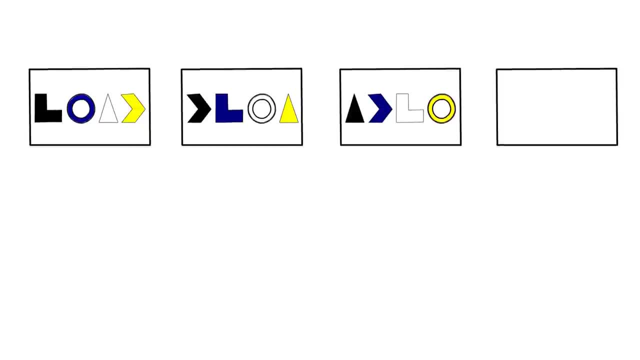 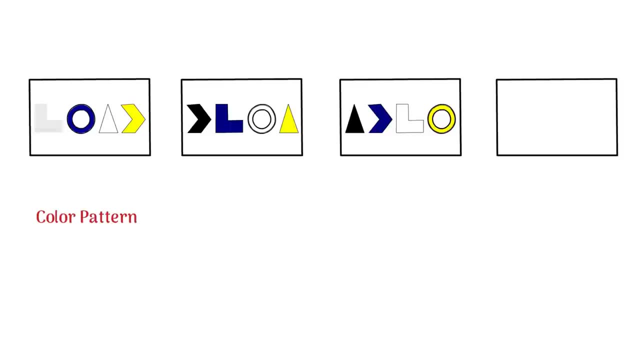 Let's continue to see how we can get to the correct solution together. In most types of problems, there are typically multiple patterns present. For example, let's look at the color pattern. If you look closely, you see that the first shape inside the rectangle 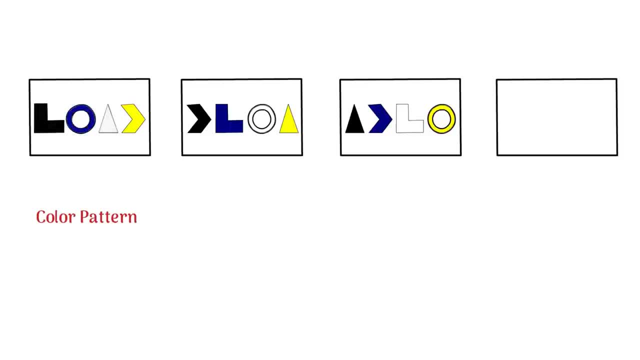 is always black, second shape is always purple, third shape is always white and the rightmost shape is always yellow. The second pattern that you can see if you look closely is the pattern of rotating shapes. You can see that the rightmost shape 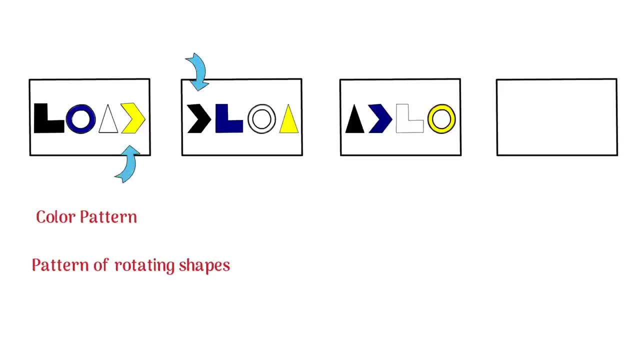 in the previous rectangle always becomes the leftmost shape in the next rectangle. For example, the yellow arrow from the first rectangle becomes the black arrow in the second rectangle. If you are able to identify at least one of these patterns, you will be able to solve this problem. 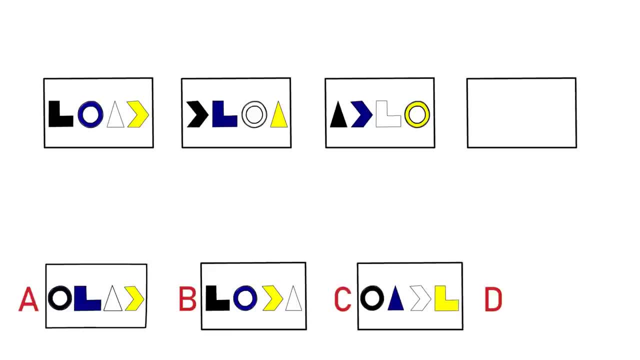 Let's look at each of the answers and try to exclude the incorrect answers. For example, choice A does match the color pattern, but if you look closely, the next shape after the circle should be triangle and not the L shape as it is currently presented in the choice A. 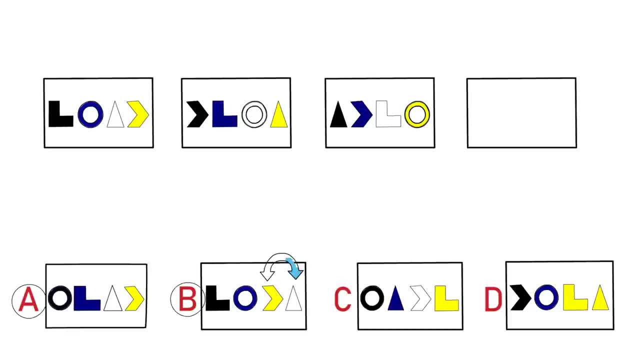 Choice B can be excluded because it doesn't match the color pattern. As you can see, the yellow shape and white shape should be swapped to match the color pattern. Choice C is the correct answer. It does meet requirements for both patterns, And choice D does not match the color pattern. 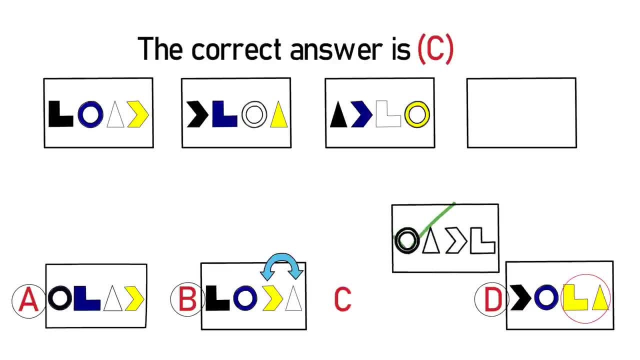 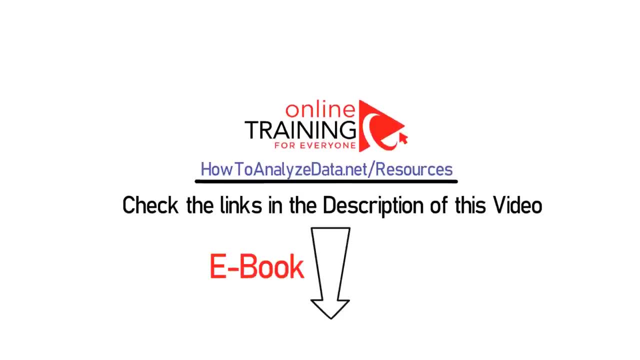 Two rightmost shapes are yellow. Hopefully you've nailed this question and now know how to answer similar problems on the test, But in case you need more questions like this, please make sure to check out my ebook in the description section of this video. 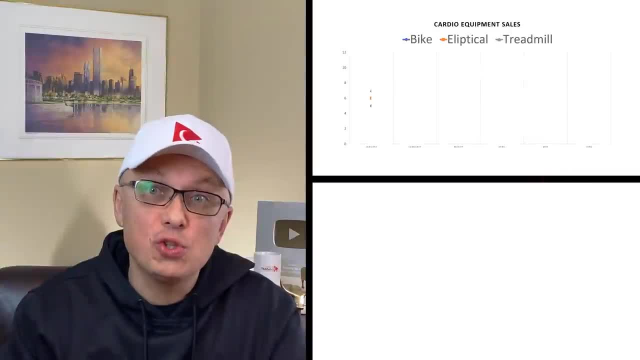 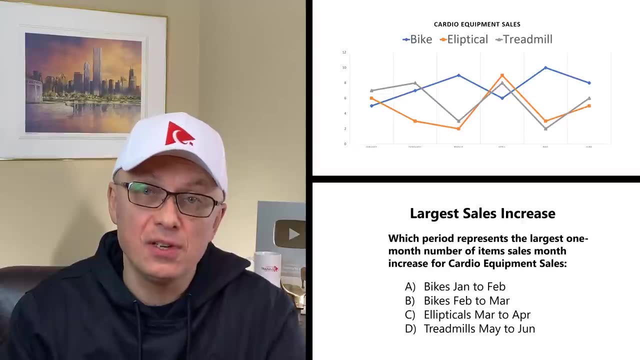 A lot of times you might get a question which asks you to determine the sales increase. You're typically presented with the graph, which shows lines that represent different sales. In our case, we are represented with the chart that shows sales of cardio, which represents different sales. 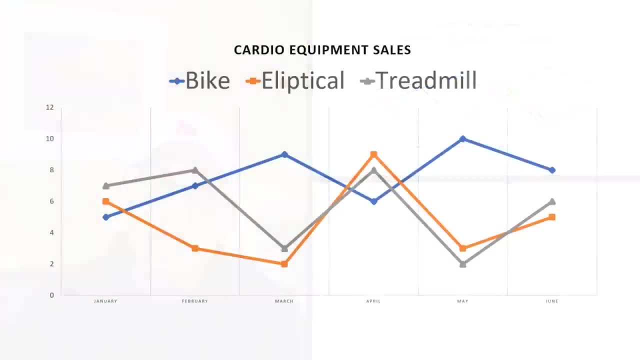 In our case, we are represented with the chart that shows sales of cardio, which represents different sales From January to June, sales of bikes, represented by the blue line, sales of elliptical, represented by the orange line, and sales of treadmills are represented by the gray line. 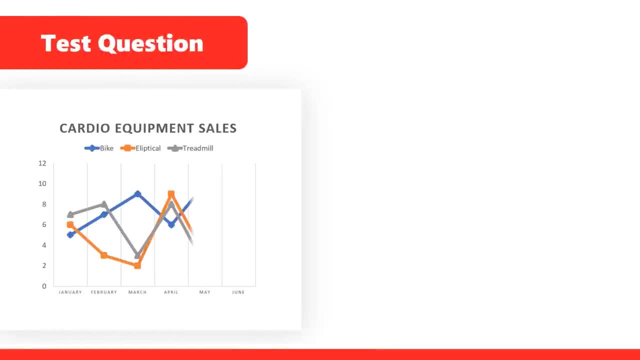 The question asks you to determine largest sales increase. Specifically, you need to determine which period represents the largest one month's number of item sales increase. for cardio equipment sales. You have four different choices. Choice A bike, which represents the largest sales increase. 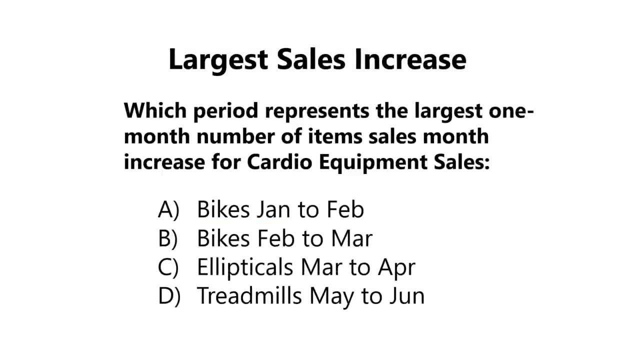 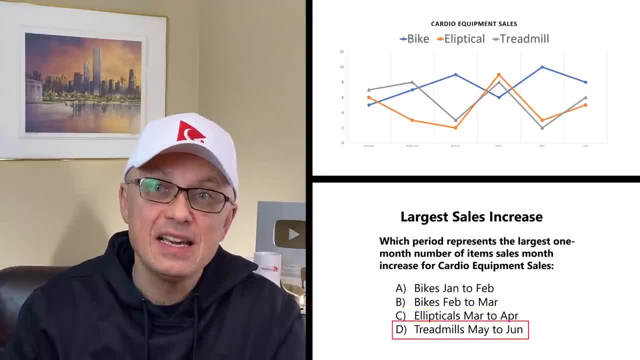 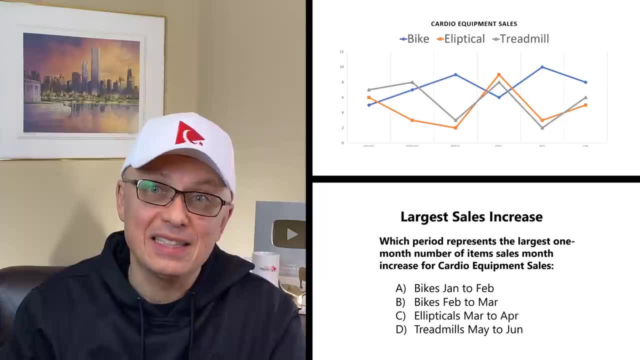 Choice B bike, which represents the largest sales increase. Choice B bike, which represents the largest sales increase. Choice C ellipticals in March to April. Choice D treadmill in June. Do you see the answer? You might need to look closely to determine the correct answer for this question. 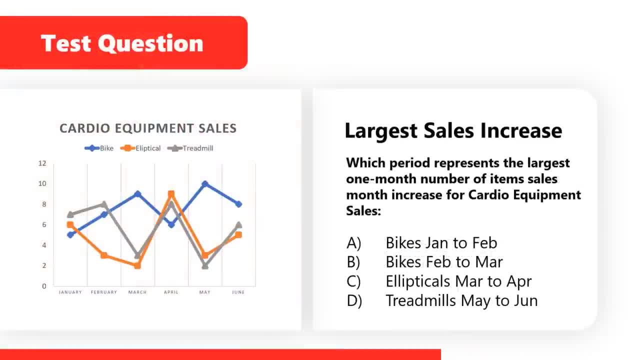 Give yourself 5-10 seconds to see if you can come up with the right solution. Are you ready? We're going to move forward and cover the answer for this problem and get to the solution together. We're going to move forward and cover the answer for this problem and get to the solution together. 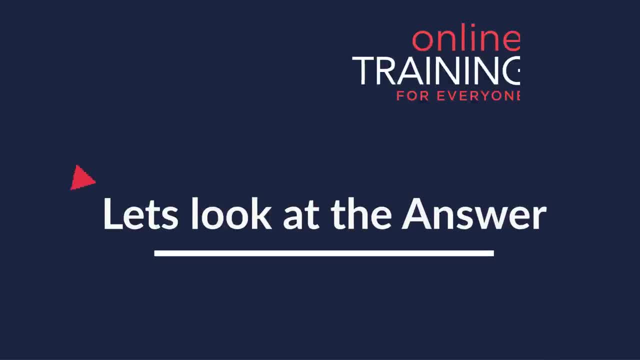 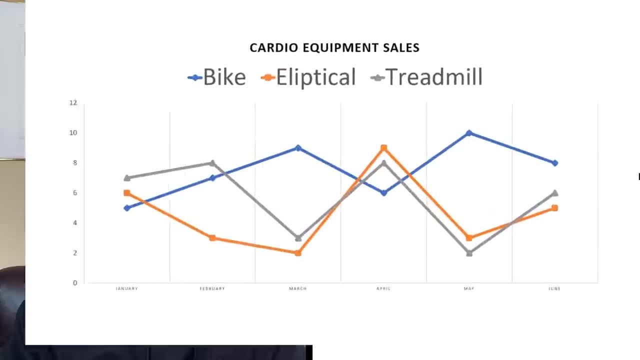 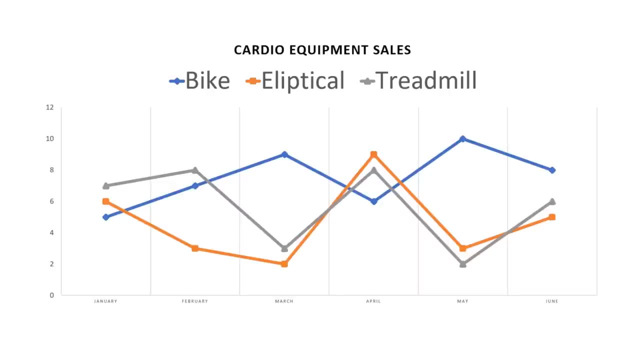 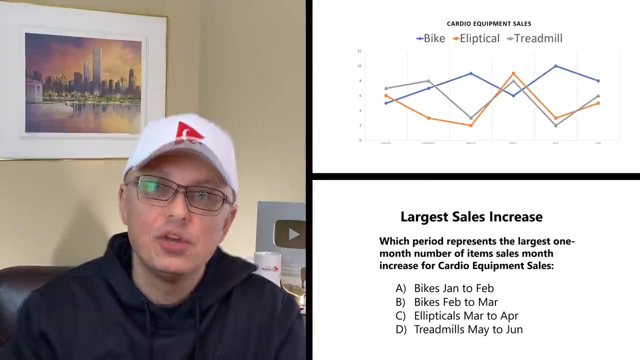 To answer this question, we need to look at the graph closely. For each data point on the graph, we need to determine the actual value And once we have all the numbers, we need to answer the question by looking at the differences for equipment sales from month to month Specifically. 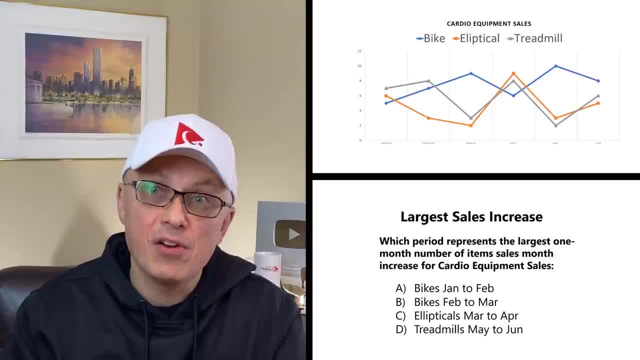 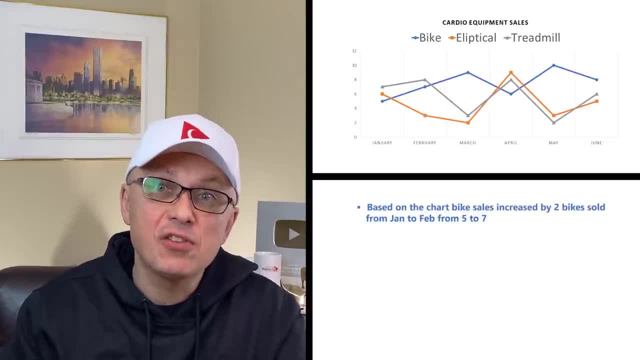 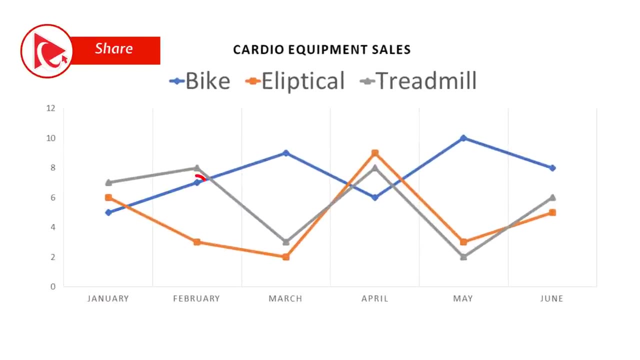 in this case, you need to evaluate four different choices that are represented by answers A through D. Let's do it together. Based on the chart, bike sales increased by two from January to February and the increase was from five to seven items sold. Bike sales also increased by two from seven. 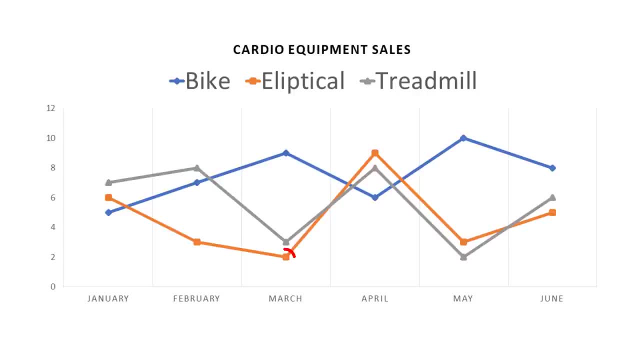 to nine between February and March. Elliptical sales, on the other hand, increased by seven from March to April, jumping from two to nine, And treadmill sales increased by four between May and June, going up from two to six. So the 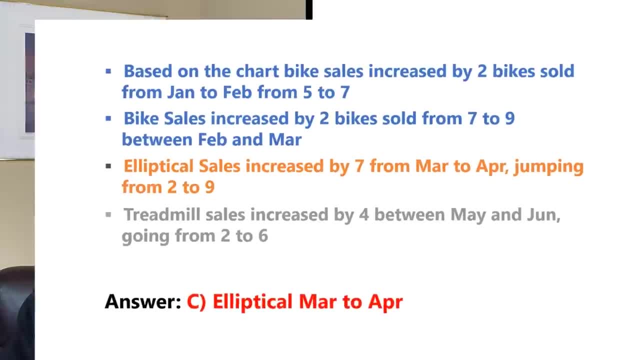 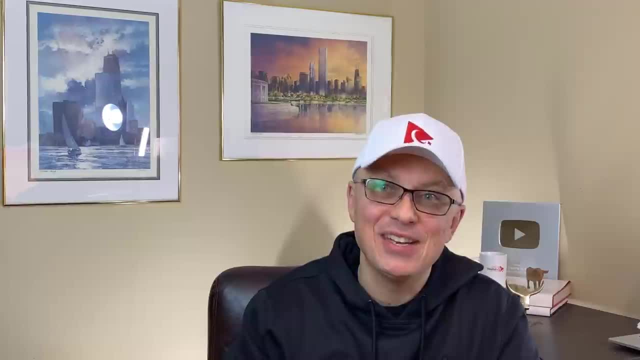 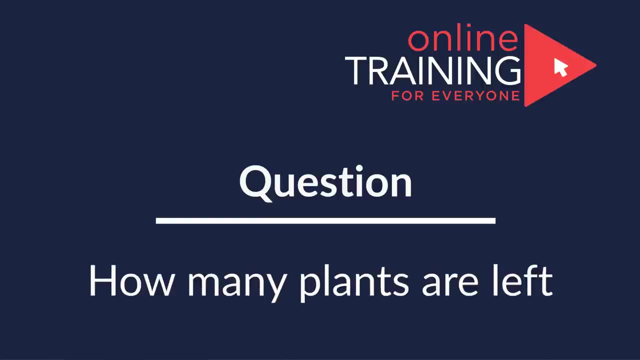 correct answer here is choice C: elliptical sales from March to April, because jump was by seven from two to nine. Hopefully you've nailed this question and now know how to answer similar problems on the test. I'm very excited to present you with simple. 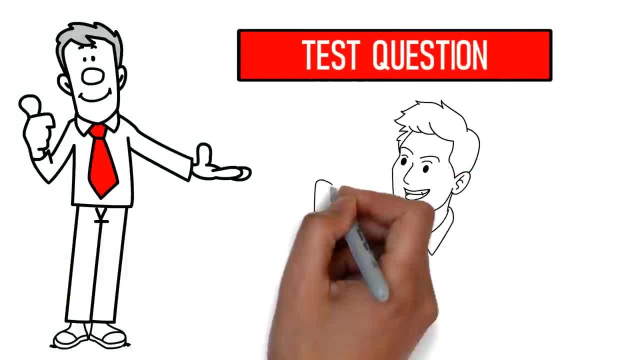 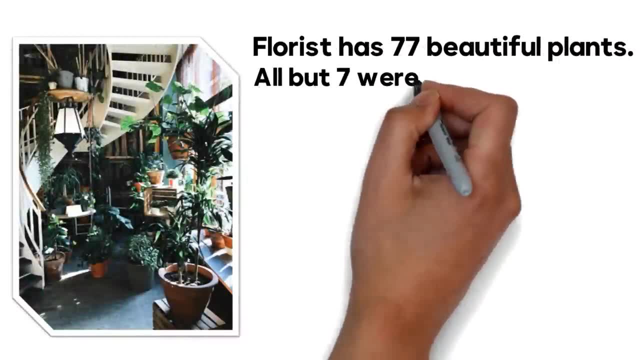 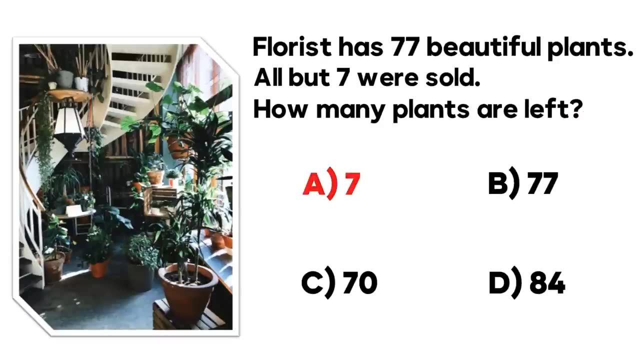 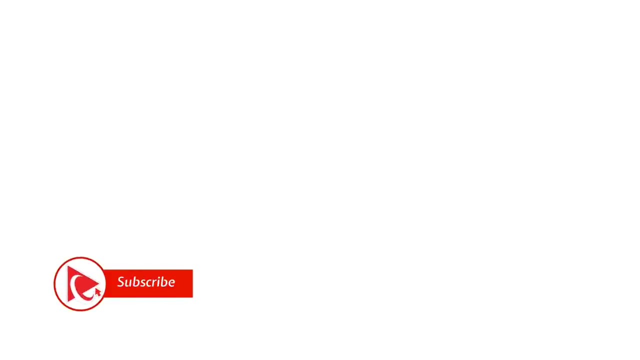 but very easy to solve questions, So let's get started. Do you think you know the answer? Let's continue to see how we can get to the correct solution together. The answer to this question is very simple: Seven plants are left. The answer is hidden. 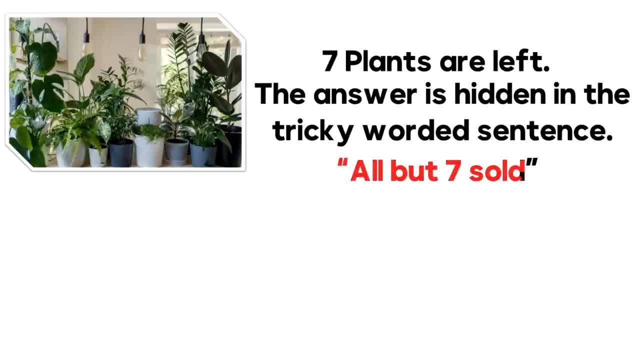 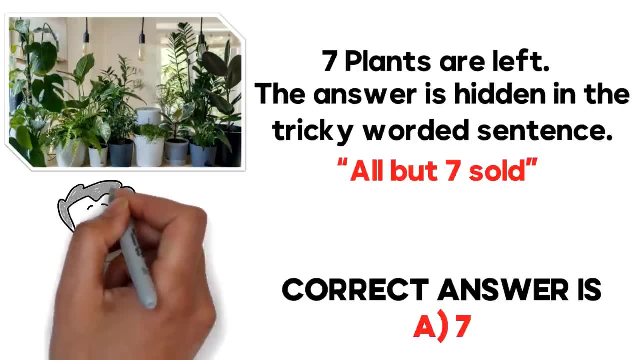 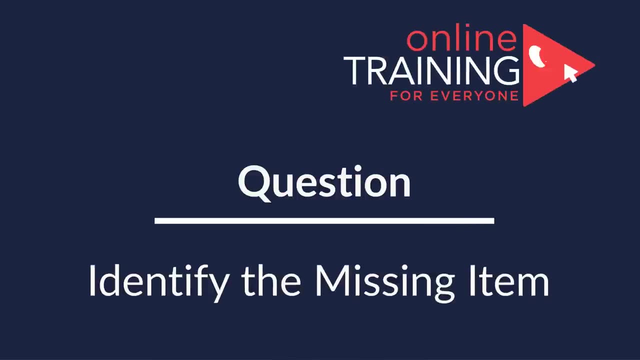 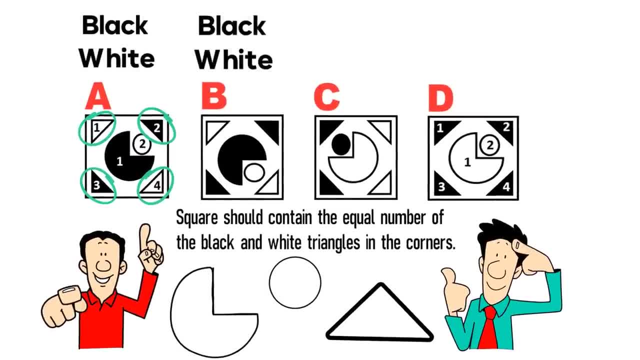 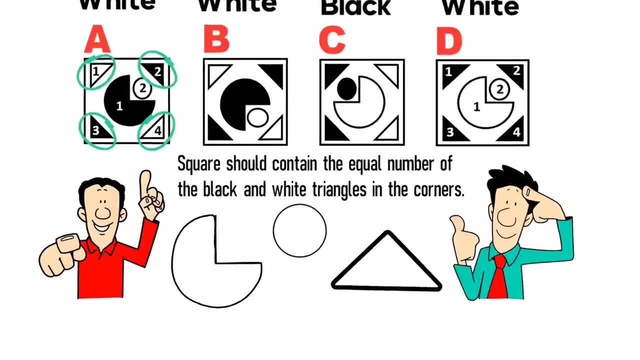 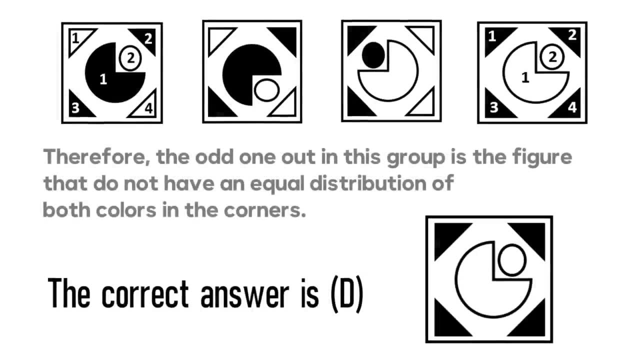 we have black- white, shape b- black- white, shape c- white- black and then shape d- white- white. based on this information about the circles, we should ignore them and focus on the triangles inside the squares. this is why the odd shape, the shape that doesn't belong to the group, is the one that does. 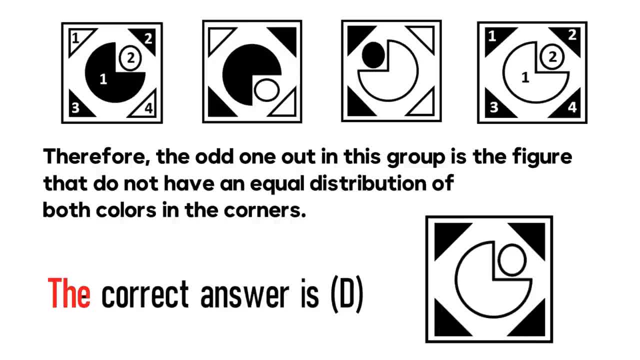 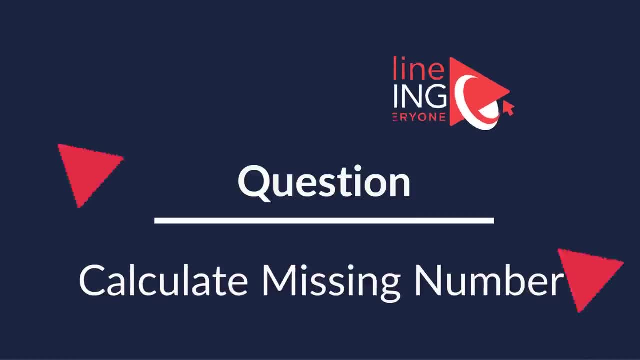 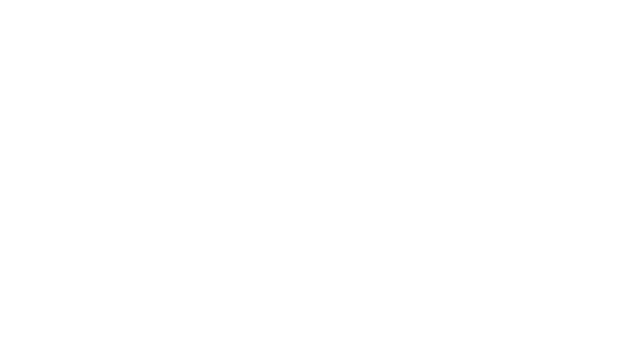 not have equal distributions of all colors in the corners, so the correct answer here is choice d. hopefully you've nailed this question and now know how to answer similar problems on the test. this is very interesting question which requires you to do calculations based on the pattern that you need to detect. you're presented with two squares. 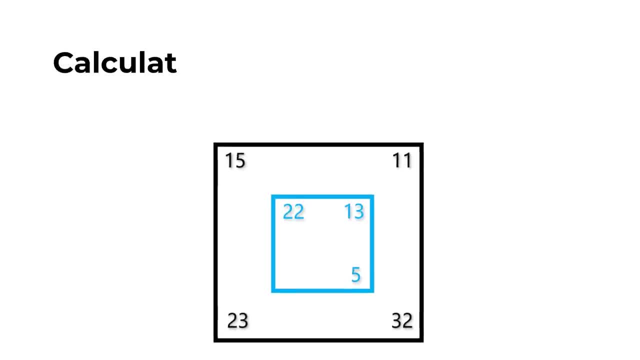 small square is located inside the larger square. there are numbers in all corners of the larger square as well as in all corners in the smaller square. if we start looking at the numbers in the upper left corner and go clockwise, you see the numbers 15, 11, 32 and 23. in the smaller square, the numbers are 22, 13 and 5, and one number is missing, and this: 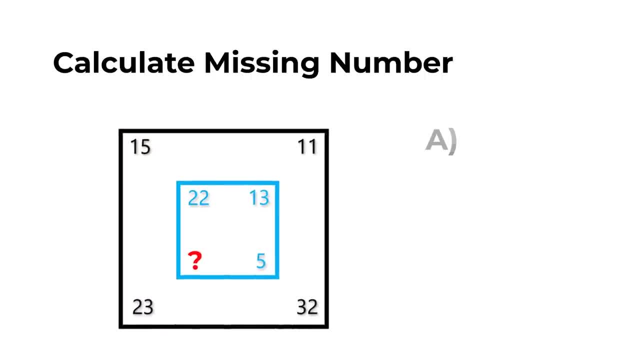 is the one that you need to calculate. your choices are: choice a: 1. choice b: 7. choice c: 12. choice d: 17.. give yourself 10 points for that question. You can also find this information in the description of this video. I'll give you the answer at the end of the video. Thank you for watching. Bye, Bye.